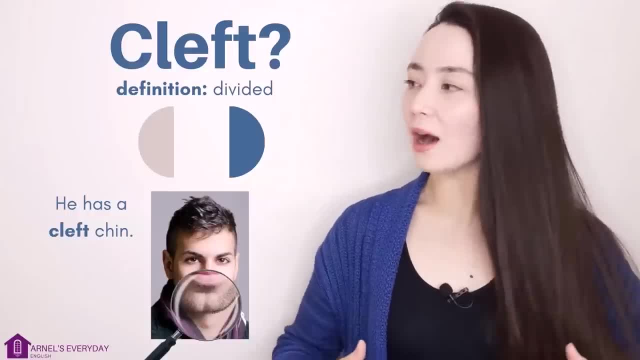 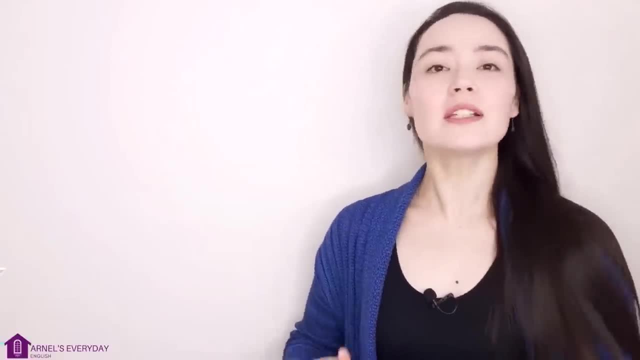 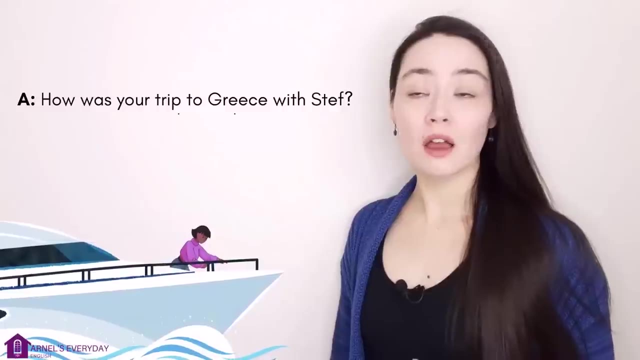 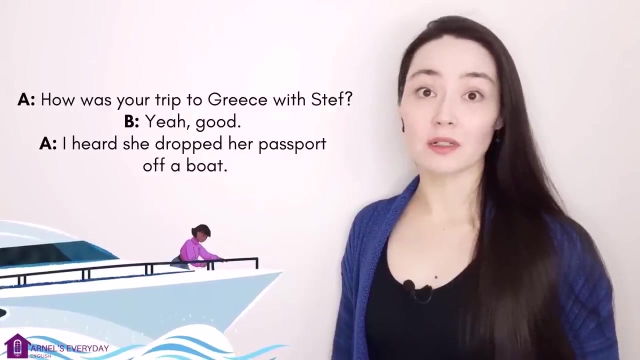 lesson: what is being divided? How does a sentence become a cleft sentence? I'll show you. Let's start with a really simple conversation. How was your trip to Greece with Steph? Yeah Good, I heard she dropped her passport off a boat, Her. 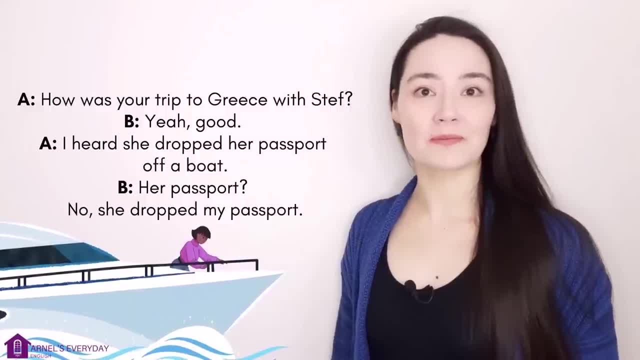 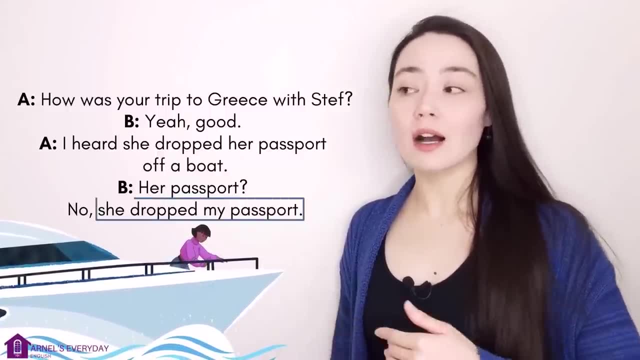 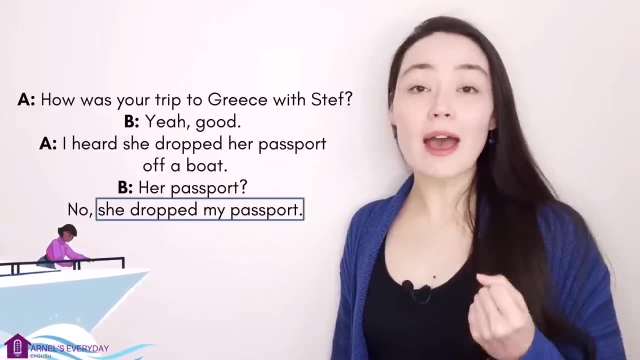 passport. No, she dropped my passport. Okay, here we have a really standard conversation. But in this last part here I'm correcting someone, right? What can I do to give a little bit more emphasis to this correction? I can use a cleft. 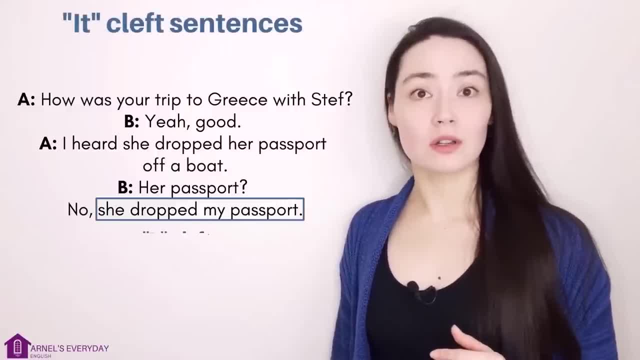 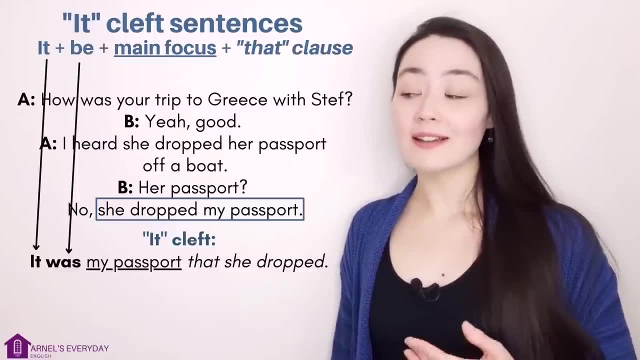 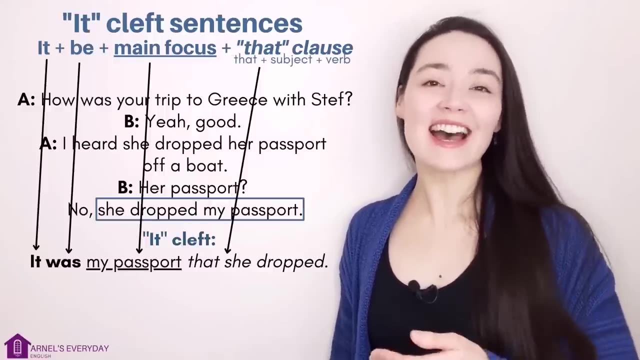 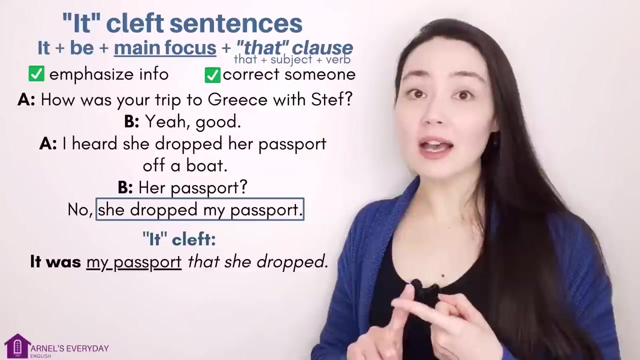 sentence: Her passport. No, it was my passport that she dropped It. B main focus: that clause. What do I mean by that clause? That's a subject verb. We use cleft sentences to emphasize information or to correct someone Of. 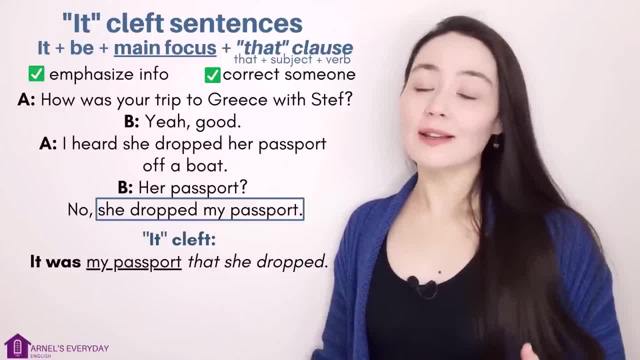 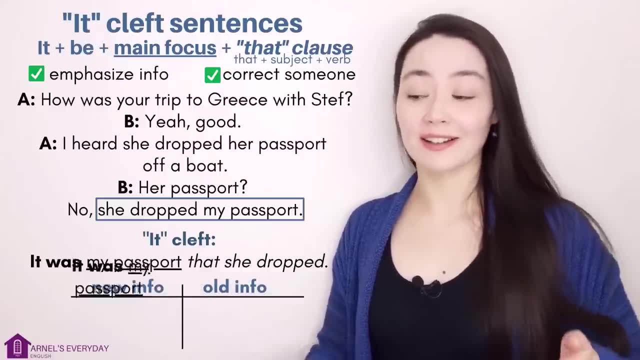 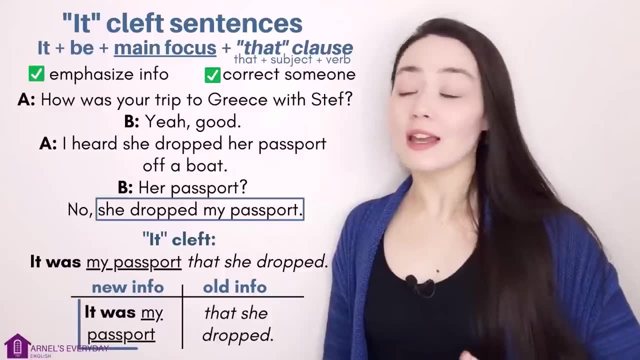 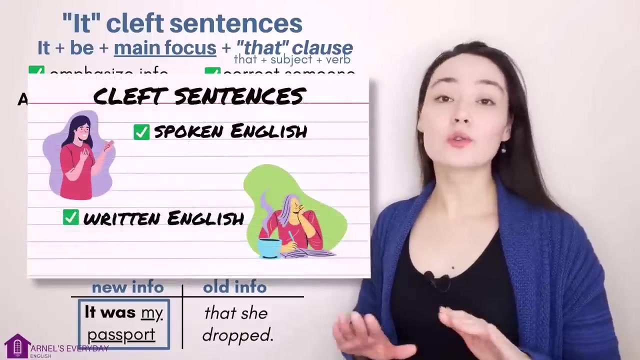 course you could just use a standard sentence, but we need variety. What's being divided here? We have new information, Old information. You can see the it part really emphasizes something. new. Cleft sentences are great in spoken English, but you'll see them a. 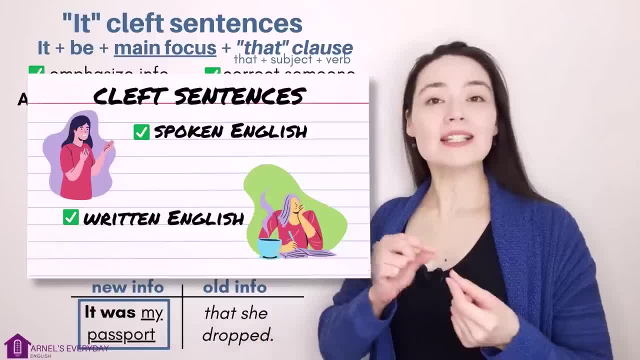 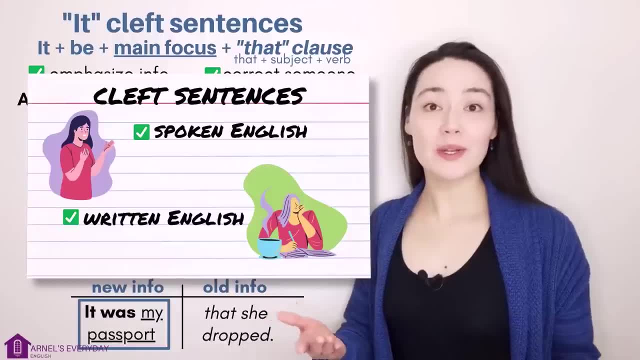 lot in written English. Why? Because in writing you can't emphasize things with your voice or your facial expressions. So what can we do? We use the grammar, so keep your eyes peeled for cleft sentence when you're reading. Let's do another example. We met our client, John Bloom. 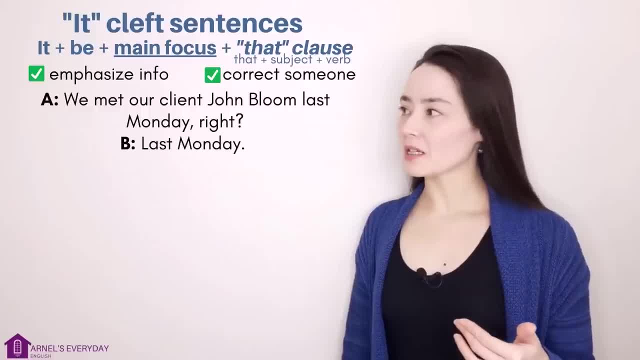 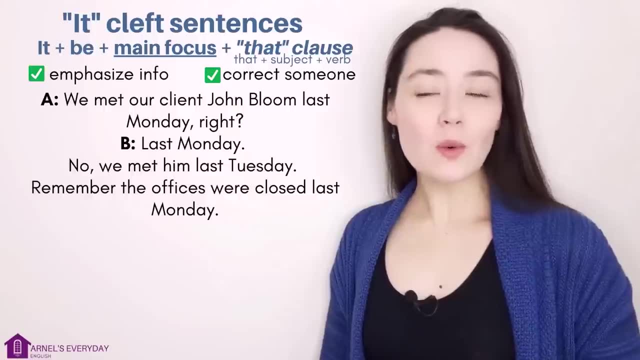 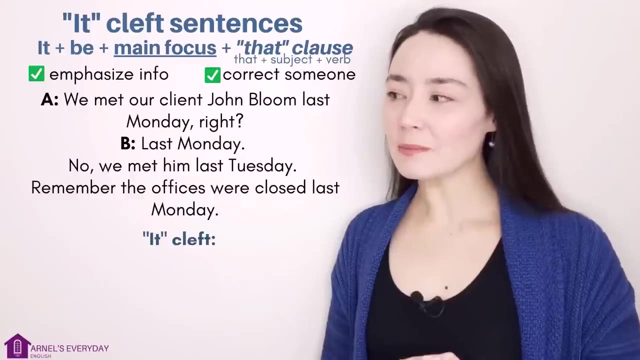 last Monday, right Last Monday. No, we met him last Tuesday. Remember, the offices were closed last Monday. What's a different way I can correct this person? How can I emphasize new information? Last Monday, No, it was last Tuesday that we. 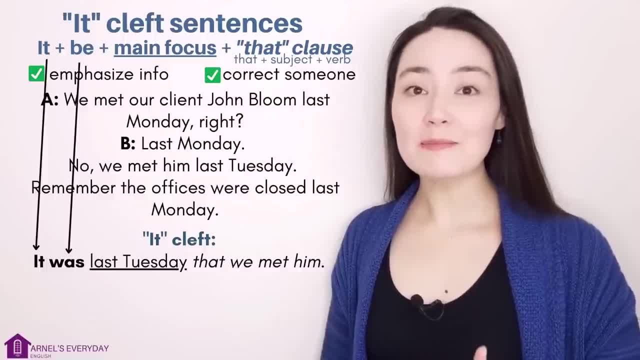 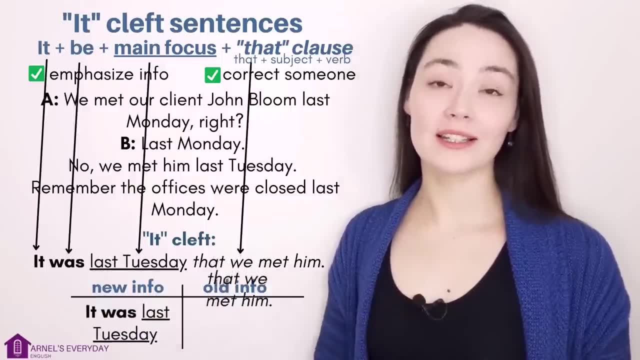 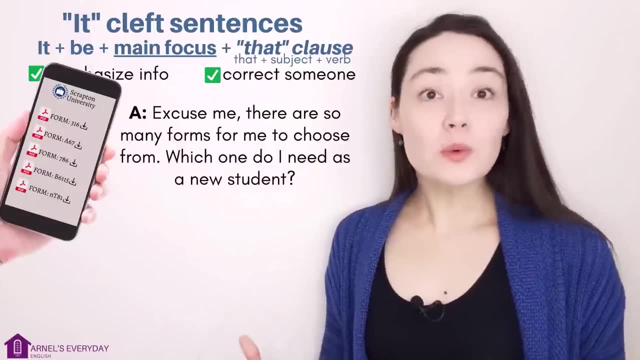 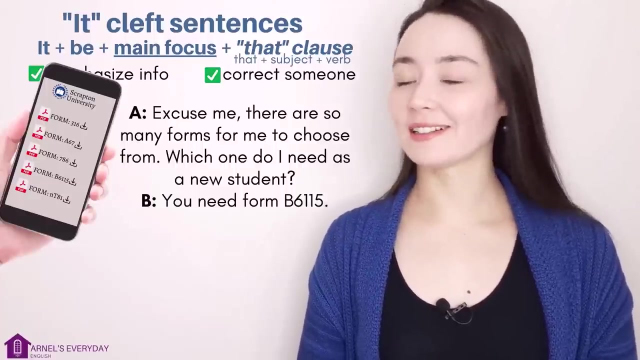 met him. It be main focus that clause. New information, old information. Excuse me, there are so many forms for me to choose from. Which one do I need as a new student? You need form B6115.. Let's make this more emphatic: It's form B6115. 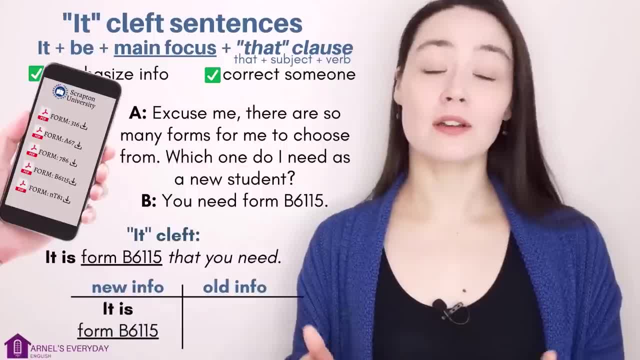 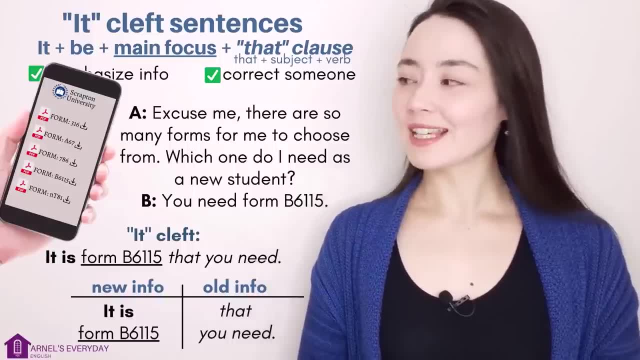 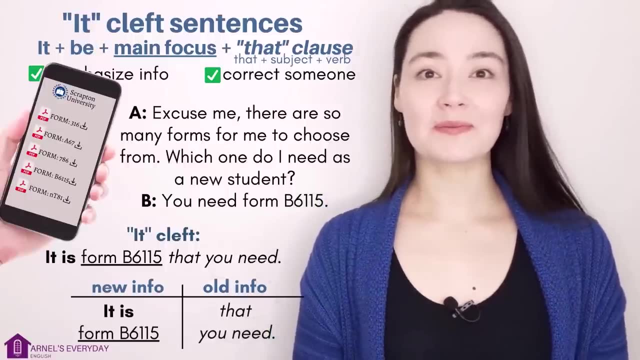 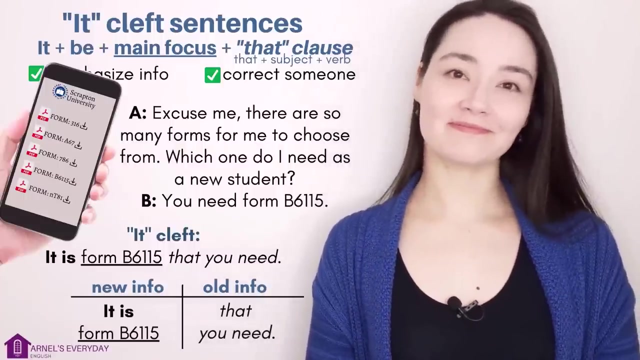 that you need New information, old, old, known or obvious information. I hope you start to get a good feeling for these it cleft sentences. Let's take this up a notch. I'm going to give you four more examples, each with a mini change. I believe it was. 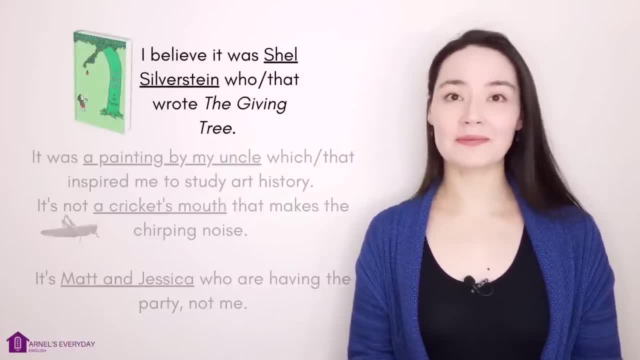 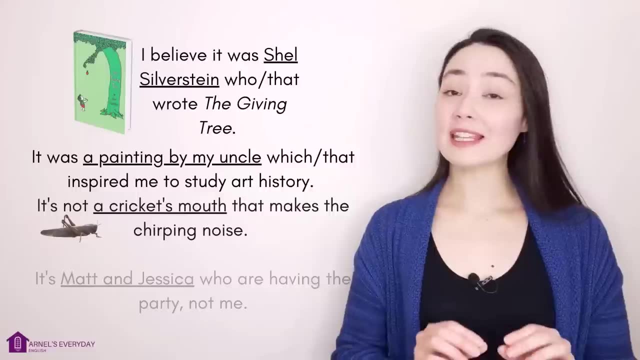 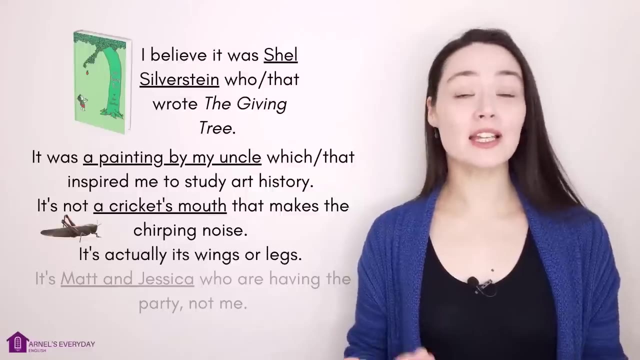 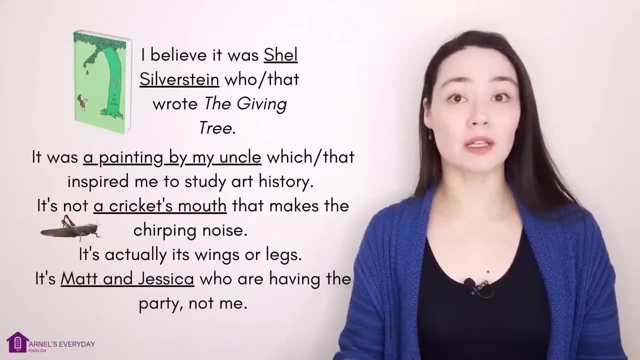 Shel Silverstein who wrote The Giving Tree. It was a painting by my uncle, which inspired me to study art history. It's not a cricket's mouth that makes the chirping noise. It's actually its wings or legs. It's Matt and Jessica who are having the party, not me. 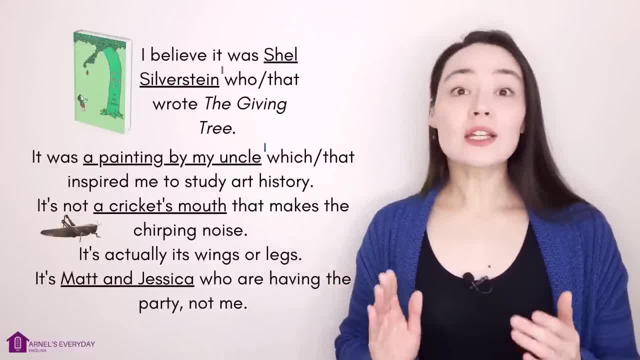 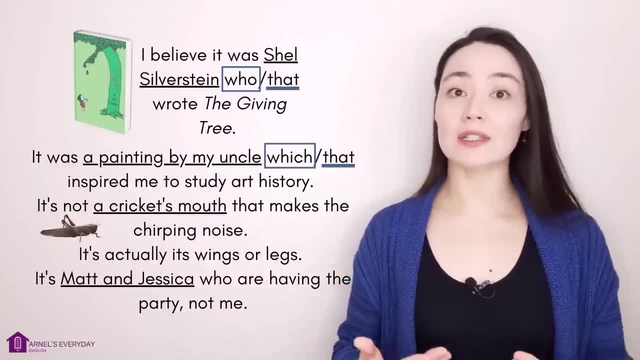 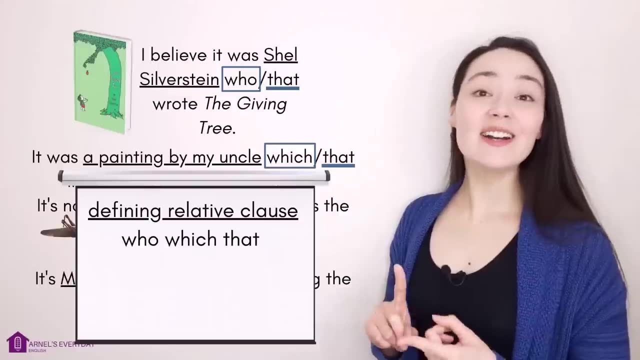 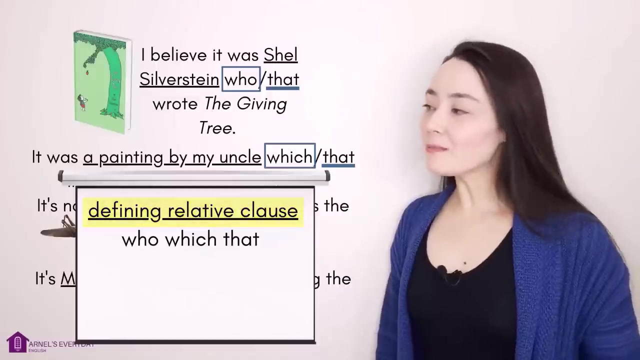 Okay, let's look at the first two sentences. You can see I've used a different relative pronoun. That is really common in cleft sentences, but we can also use who or which. Who, which or that are part of what we call defining relative clauses, And you might think 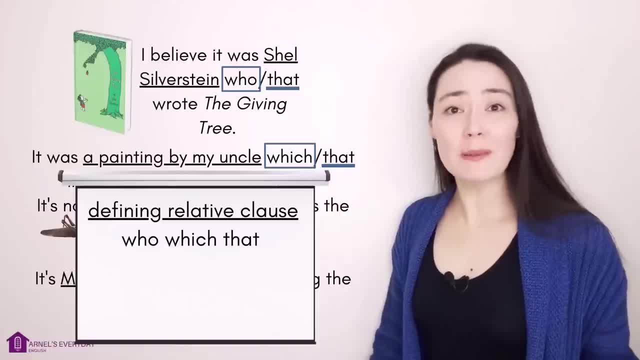 oh, defining relative clauses. what more grammar terminology For today's lesson. you do not need to be a pro on this topic, But I want to give you a little bit of information. I'm going to give you a little bit of information. 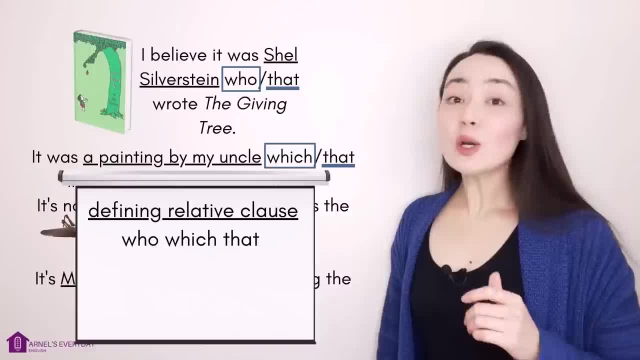 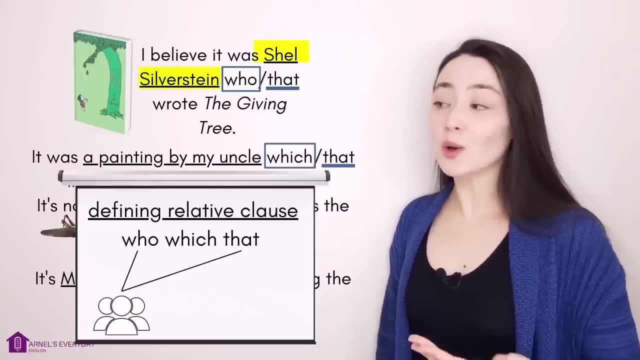 I'm going to give you a little bit of information. I'm going to give you a little bit of information. I want to give you a little reminder. We can use who or that to give more information about a person. Shel Silverstein is a man, so I can use who. 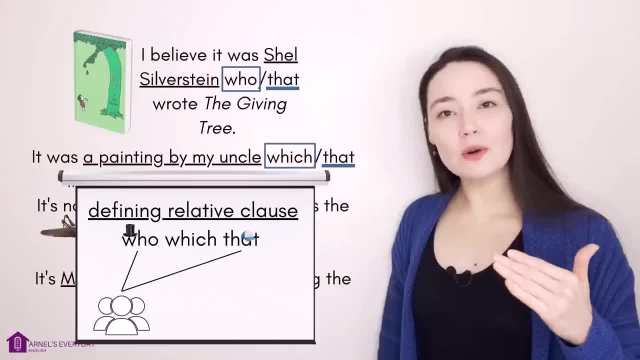 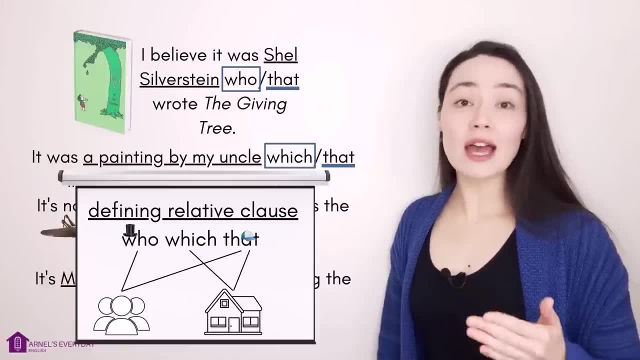 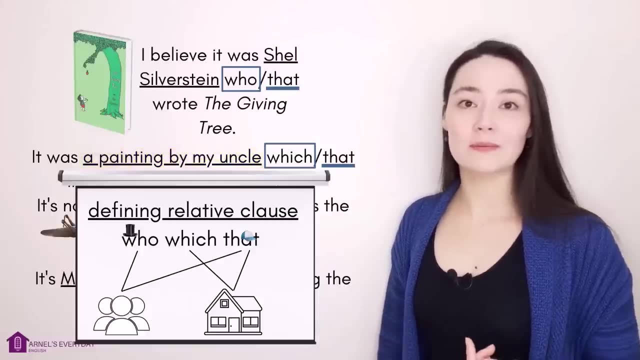 Who is a little bit more formal, that is a little less formal, but people really use these two interchangeably. We can use that or which for things, A painting by my uncle, that's an object, So I can use which, Which is a little bit more formal, that is a little bit less formal, but 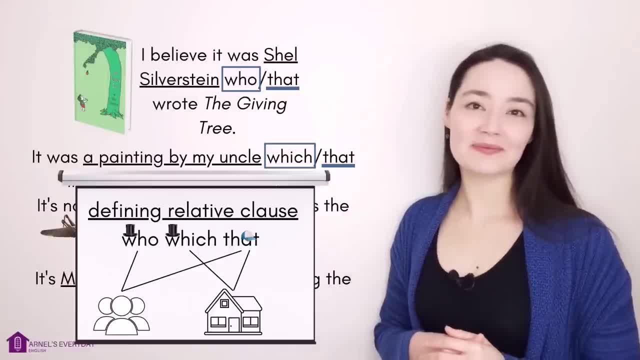 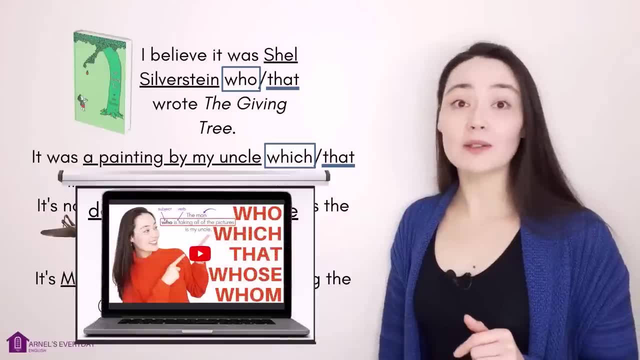 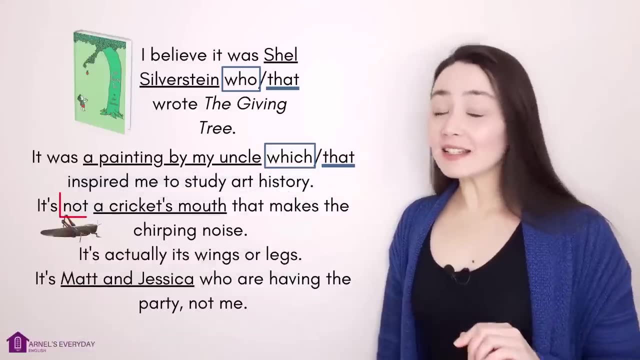 again. people use these two interchangeably. I do have a complete lesson on relative pronouns and defining relative clauses on my YouTube channel. I'll leave a link down below for you. In sentence number three, I just wanted to show you that we can also make the sentence negative. 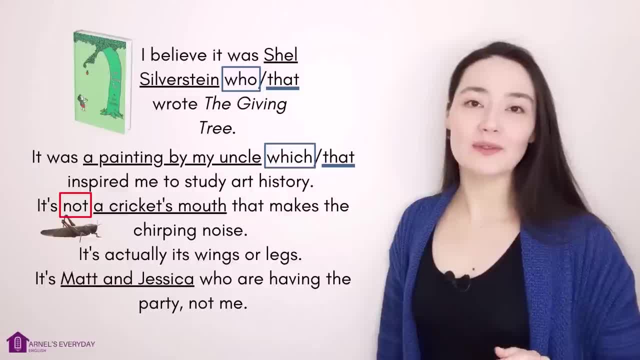 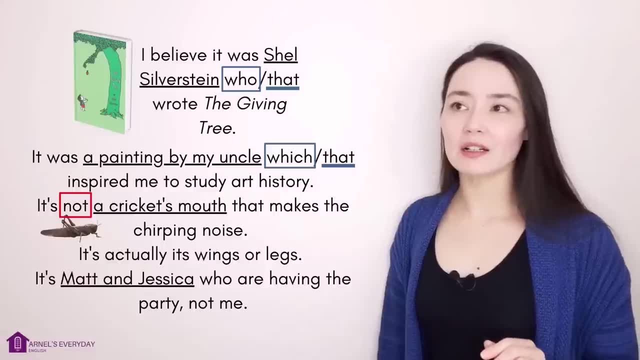 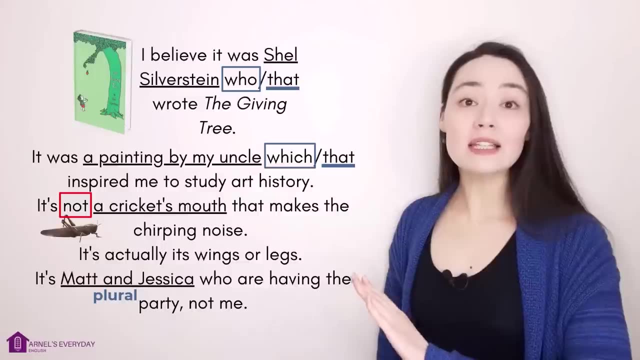 It's not. I added not there, perfectly fine. I added not there, perfectly fine. Sentence number four: Matt and Jessica, that's plural. It doesn't matter if you have a plural in the sentence, You still need a singular be after it. 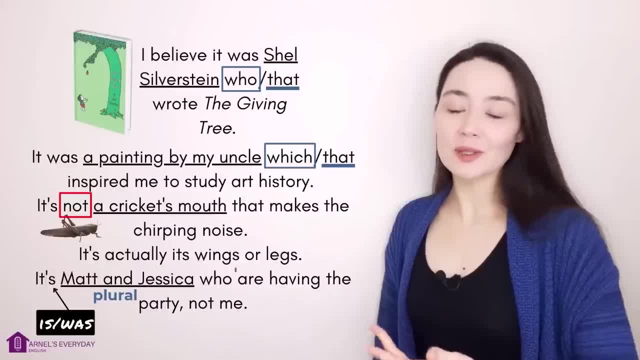 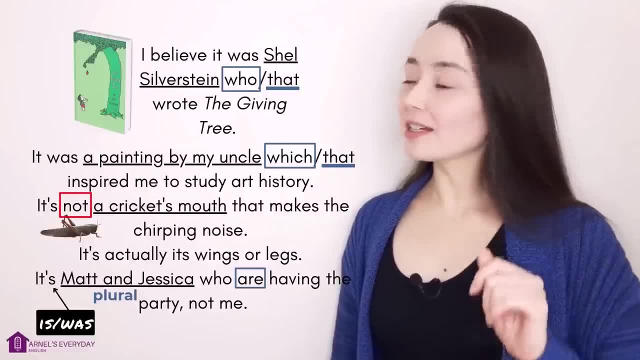 It is or it was. But in the relative clause we can use that plural verb. Here are Or maybe we're. Okay, Are we done with plural? Are we done with plural? Are we done with plural It? cleft sentences: Not quite. Let's keep going. 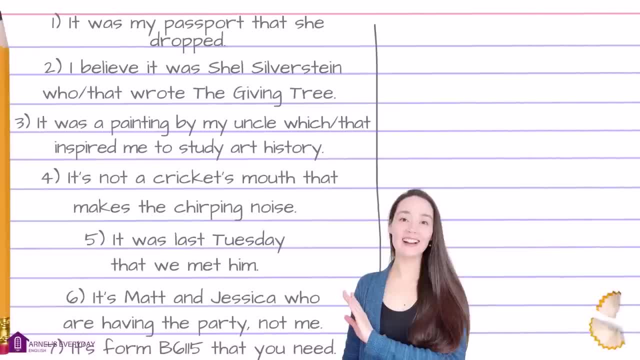 Here we have a mix of the sentences we looked at earlier in this lesson. I have my relative pronouns. Hmm, which relative pronouns can I remove? We often remove a relative pronoun in informal situations If it's the object of the verb. 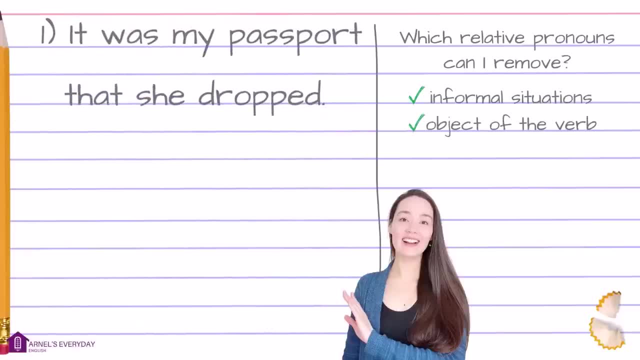 What do I mean? Let's look at sentence number one. I have my that clause. What's the verb here? Drop? What's my subject of this verb? She? What did she drop? The passport, And the passport is the object of my verb. 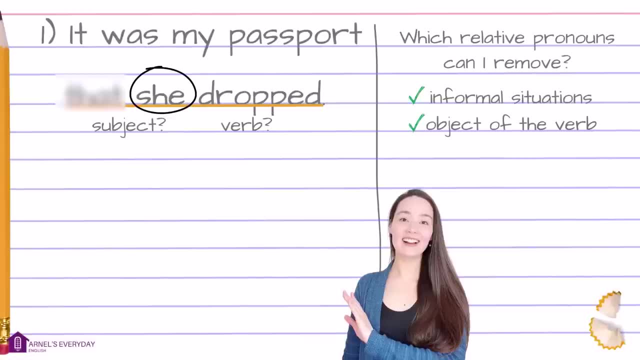 So here I do not need that. It was my passport she dropped, Perfectly correct. Let's look at sentence number two. Who wrote the giving tree? My verb is wrote. What's the subject of this verb? Here is Shel Silverstein. 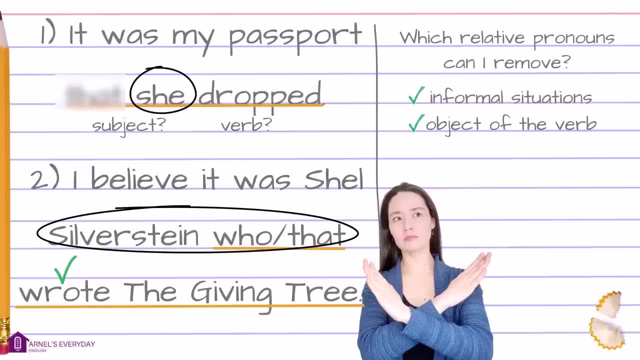 So I cannot remove who, because that's my subject. I cannot say it was Shel Silverstein wrote the giving tree. Here's a little trick: If you have a subject and a verb after your relative pronoun, you can remove it. If you only have a verb after your relative pronoun, you need to keep it because it's the subject. 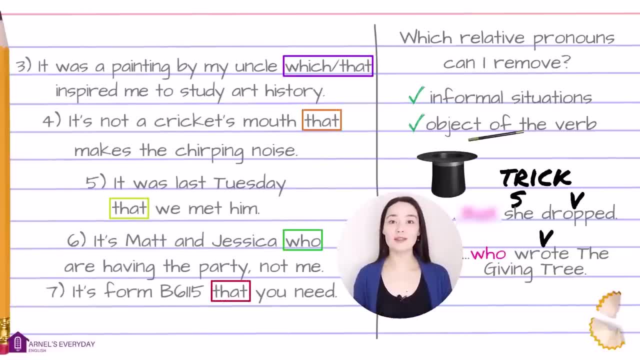 Okay, four sentences, Three, Two, seven. Decide if you can keep or remove that relative pronoun. Pause the video to do this. Okay, we can remove the relative pronoun in sentences five and seven. How do we know that? 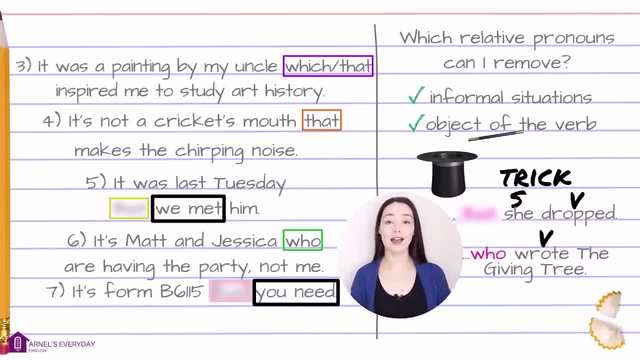 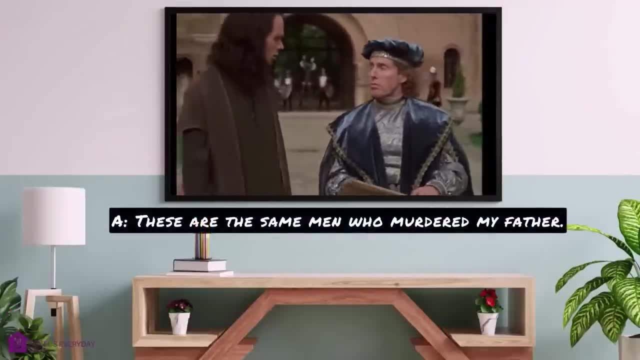 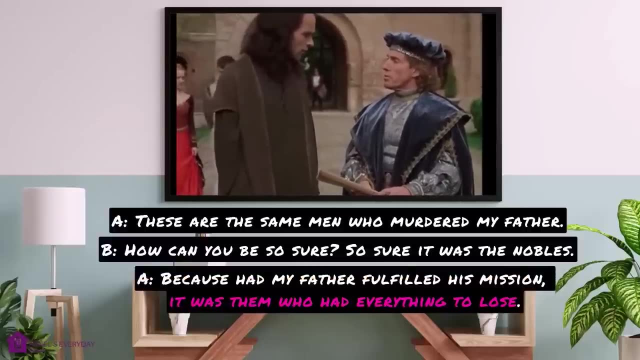 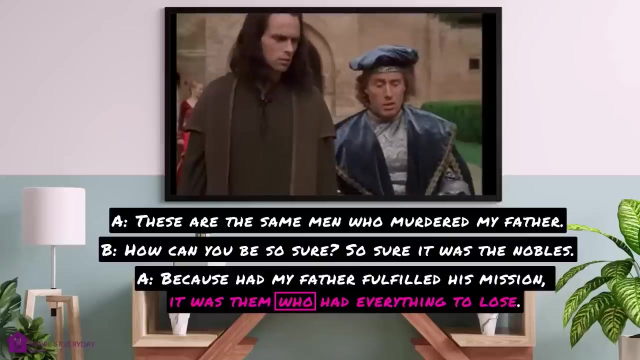 Because after the pronoun you see a subject and a verb. How can you be so sure? So sure it was the nobles, Because, had my father fulfilled his mission, it was them who had everything to lose. Is who the subject or the object of the clause? 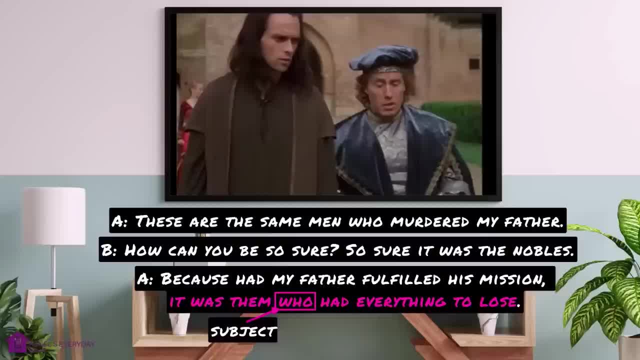 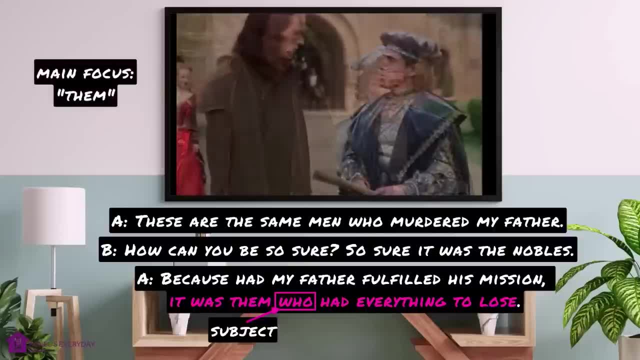 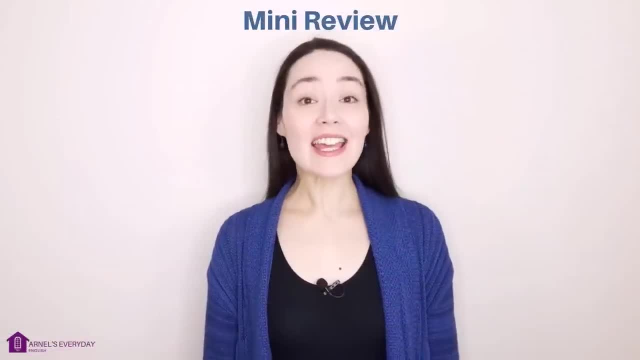 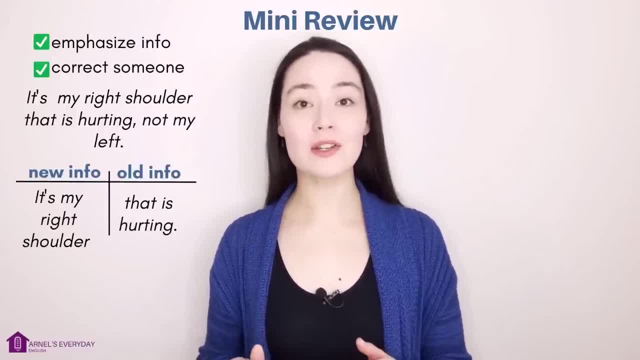 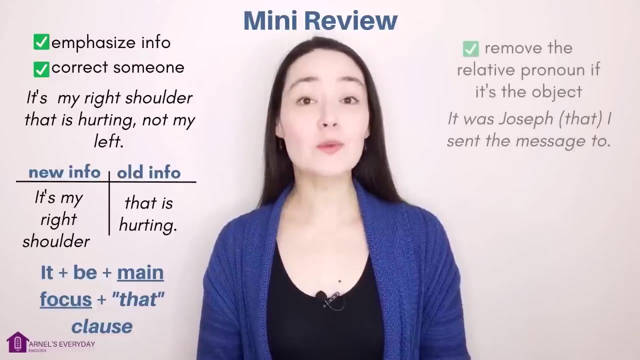 Clef sentences are divided into new information or old, obvious known information. We use a structure: It be main focus plus who which. that clause: You can remove the relative pronoun who, which or that, if it's the object. 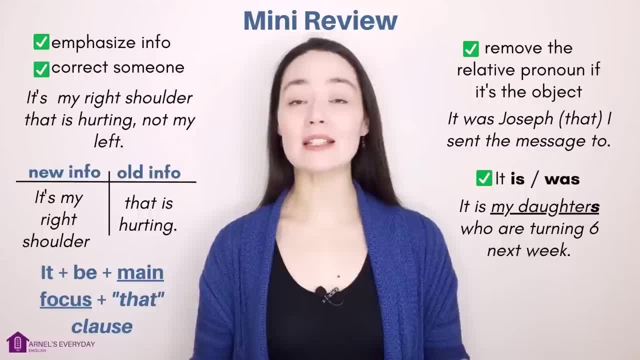 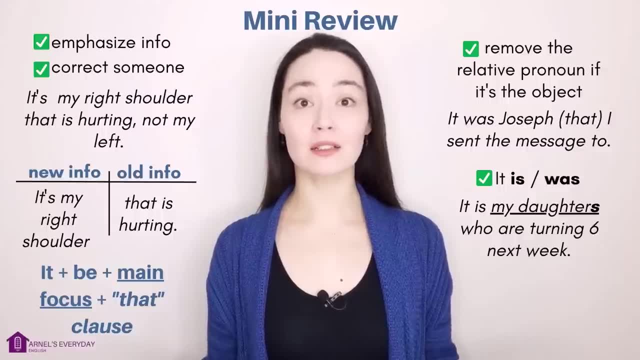 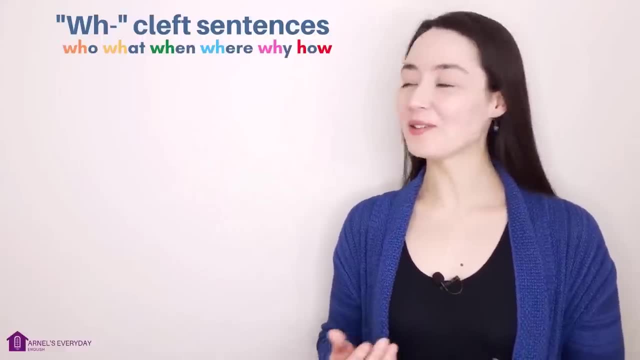 And remember after it. we always need a singular be form, Is or was. Let's keep going WH-clef sentences. What do I mean by WH? Who, what, when, where, why and how? Okay, We'll do lots of examples. 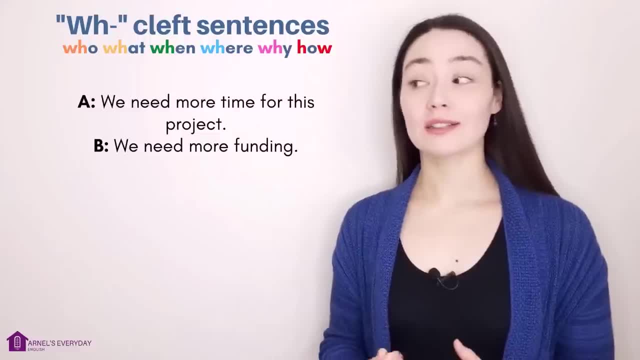 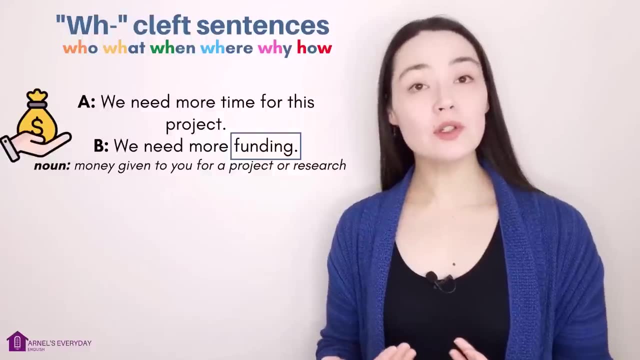 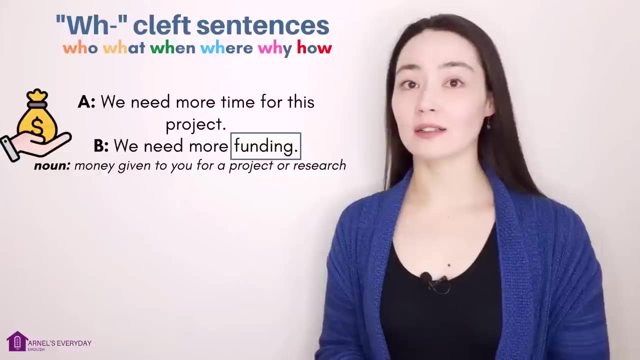 We need more time for this project. Standard sentence: We need more funding. Funding means money, Money given to you for a project or to do research. Now let's make this more emphatic. Clef sentence: What we need is more funding. 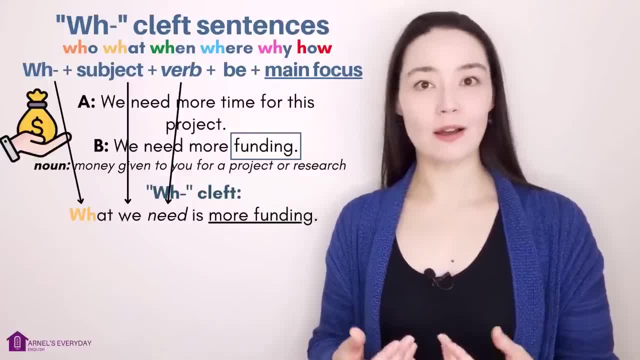 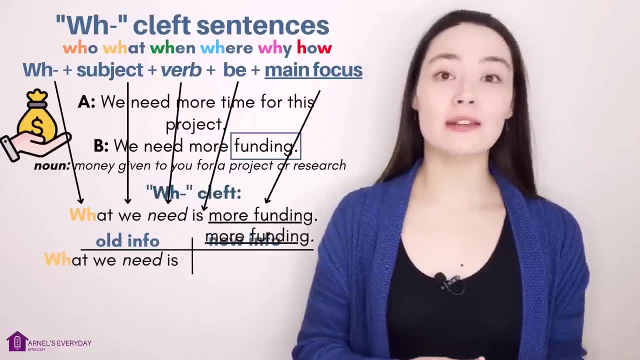 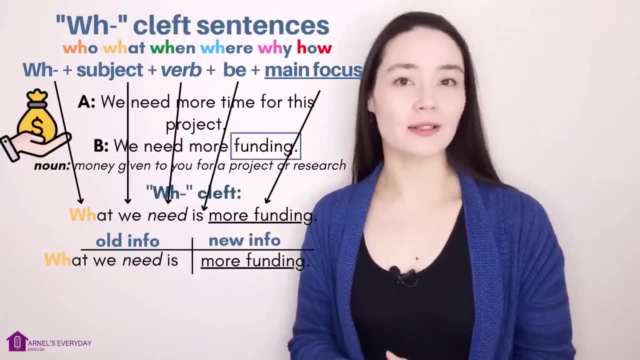 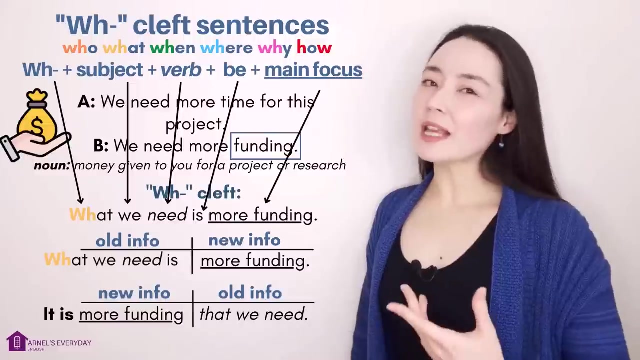 WH-subject Verb Be Main focus: Old or known information, New information. What we need is more funding. Let's compare this to an it-clef sentence just for a second. It's more funding that we need. So both of these give you the same information, but again, it's about that variety. 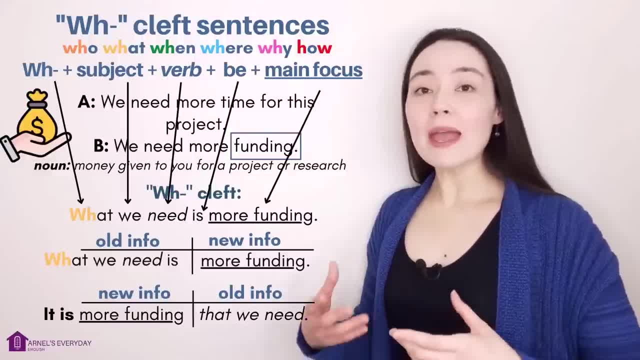 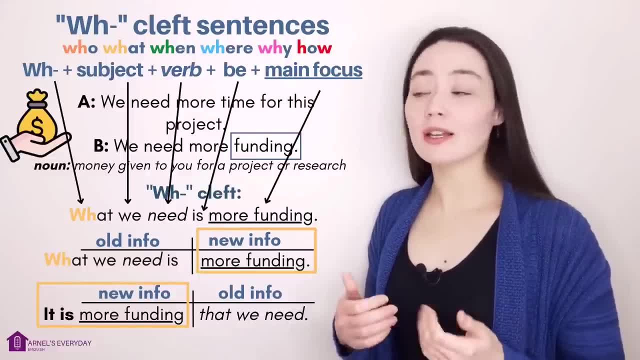 And notice in a WH-clef sentence And notice in a WH-clef sentence the main information comes from a particular tool comes at the end In an it clef sentence. that main information, that new information, comes at the beginning after it. Do you want to have some fun? We can. 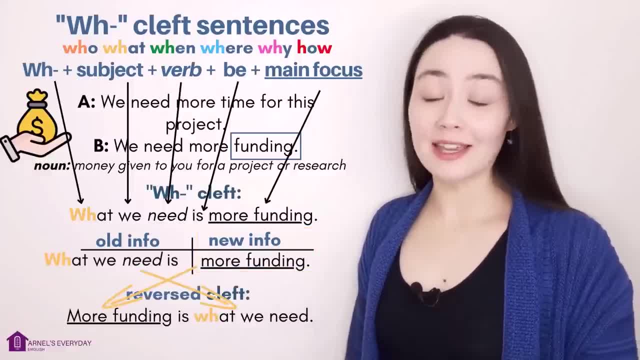 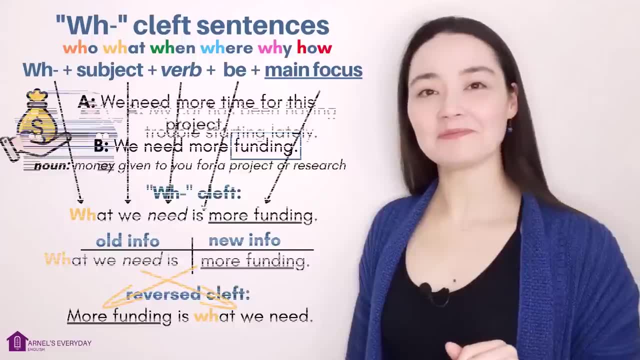 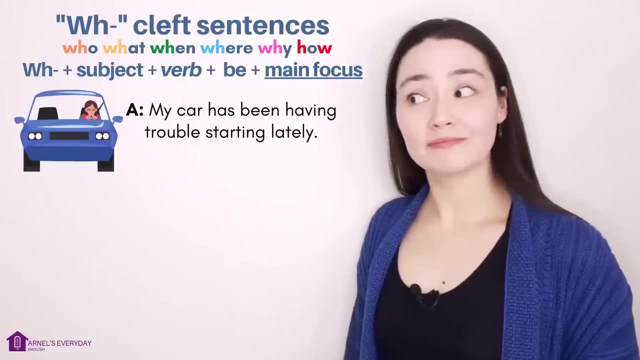 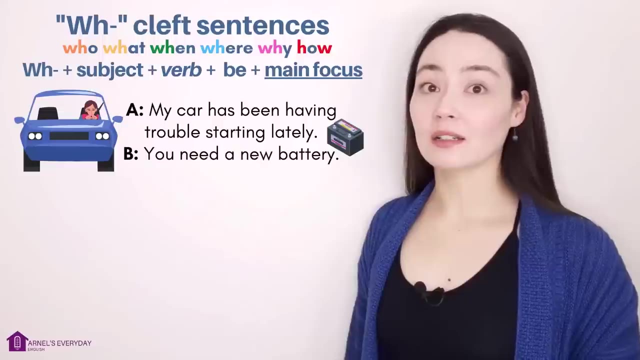 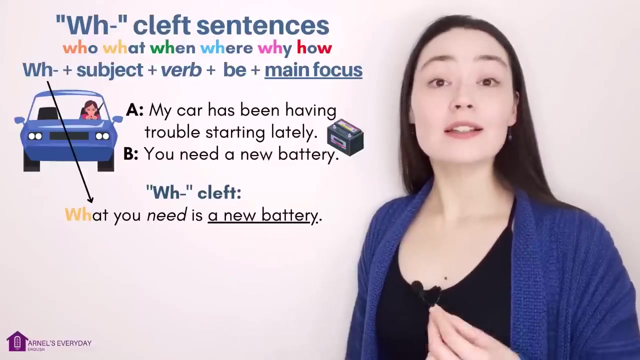 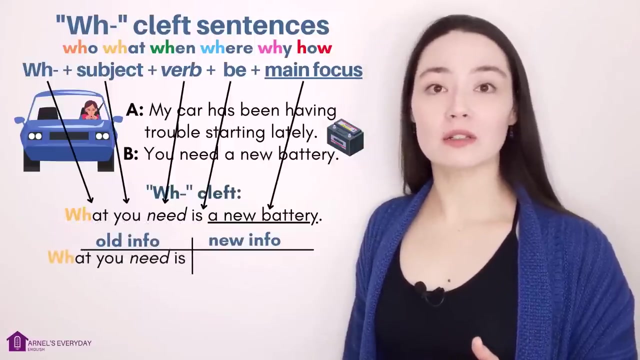 reverse the parts: More funding is what we need, Perfectly correct. Let's do another example. My car has been having trouble starting lately. Standard sentence: You need a new battery. Clef sentence: What you need is a new battery. WH Subject verb be main focus. Old information, New information. 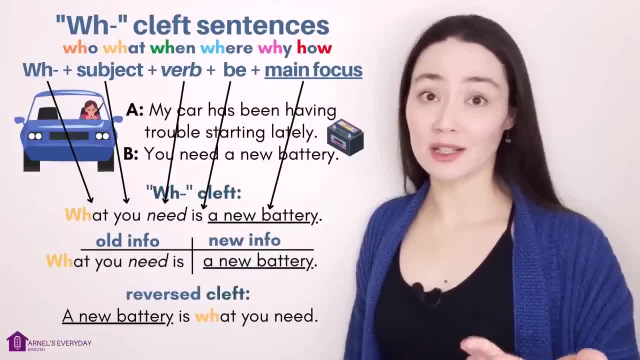 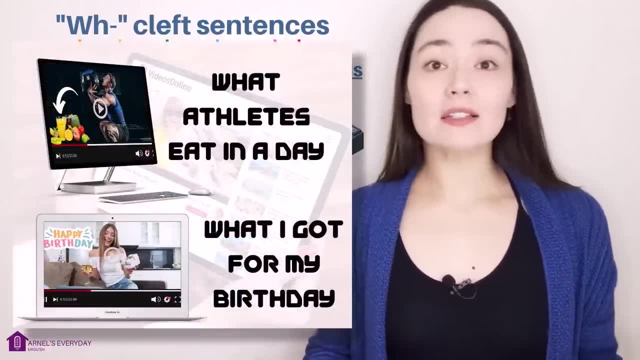 Let's reverse those parts. A new battery is what you need, and many times the matter is meant to be the same, which is why people forget to have a new battery every now and then. you'll just see the WH clause as a title of a video, For example, what athletes eat. 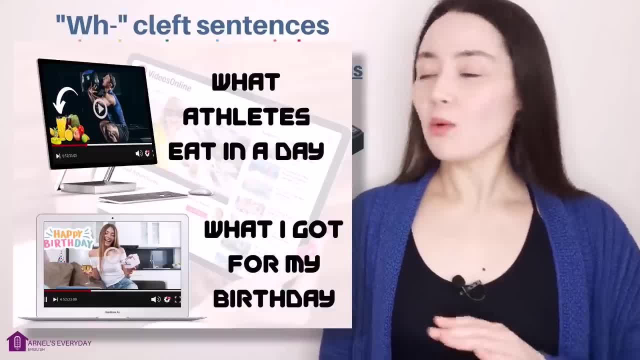 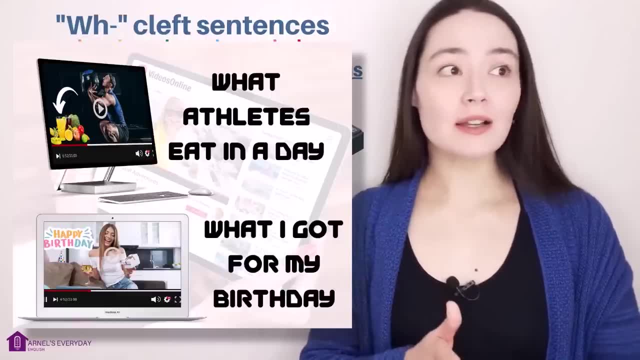 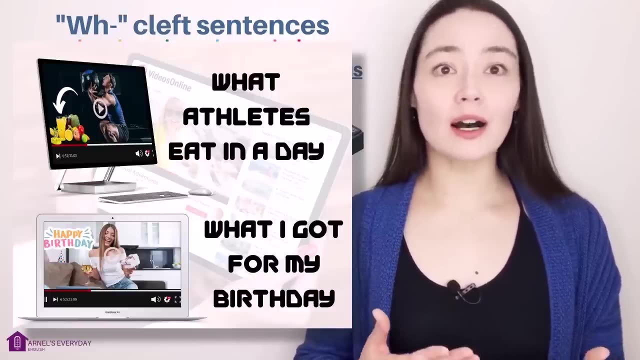 in a day or what I got for my birthday. These are just half of a cleft sentence. It's half because the main information, that new information- is in the video. So when you're looking through YouTube, keep your eyes peeled for titles like that. 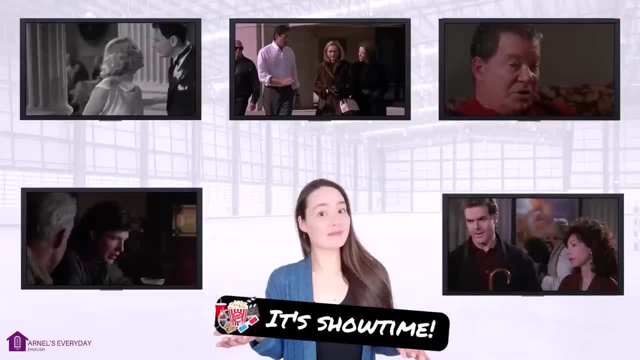 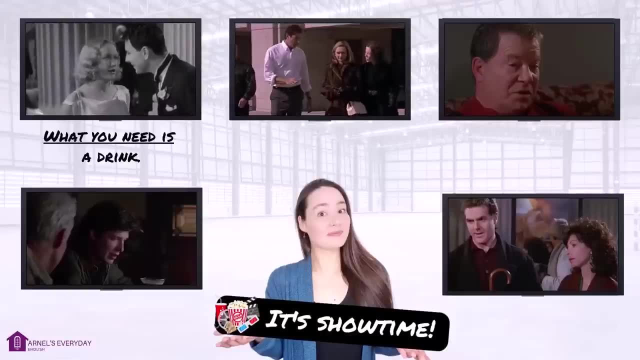 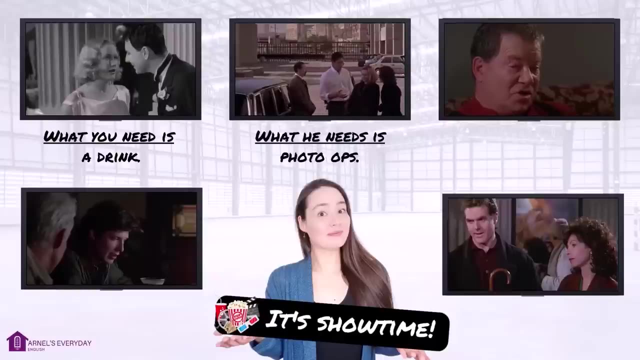 Anyway, I want to get away from here. Say: what you need is a drink, Yes, a drink. More walk, less talk. That's my motto. What he needs is photo ops Like: maybe he should plant some trees. Doesn't want to take charity, What she wants is to prove that she can make it. 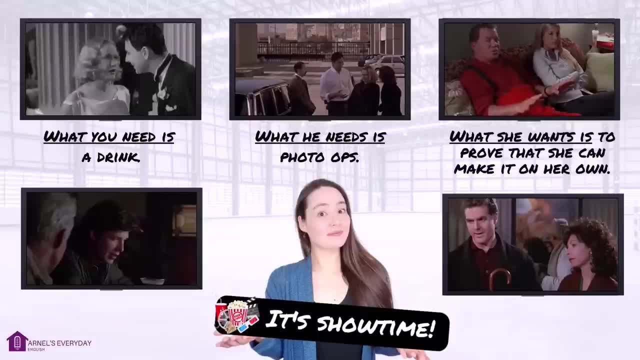 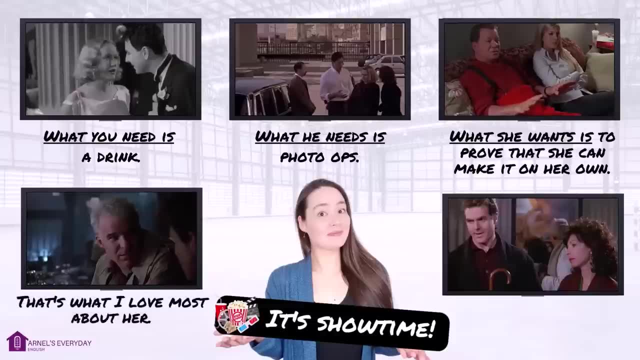 on her own. Stand on her own two feet, Earn her own. Probably one of the reasons you love Annie. That's what I love about Annie. I love most about her, That's when it hit me like a Mack truck English patient. It's just a stupid movie. That's what I'm talking about. Come on Lane, Let's go. 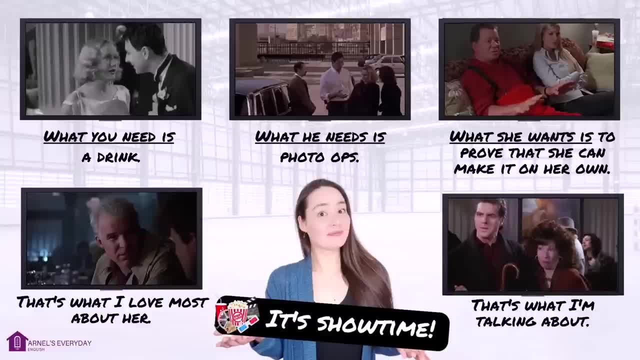 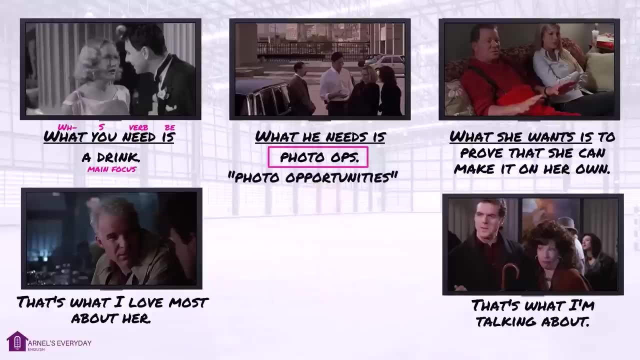 Here we have five more examples. The first example is simple: What subject verb be main focus? What you need is a drink. In the second example we can see a plural noun, photo ops, And photo ops is a word that means opportunities, Definition, A chance for people to take pictures of you so you can. 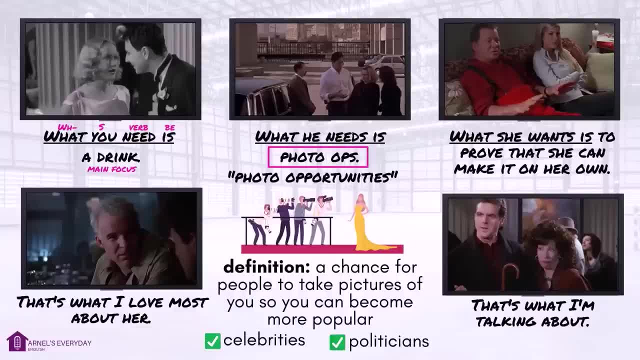 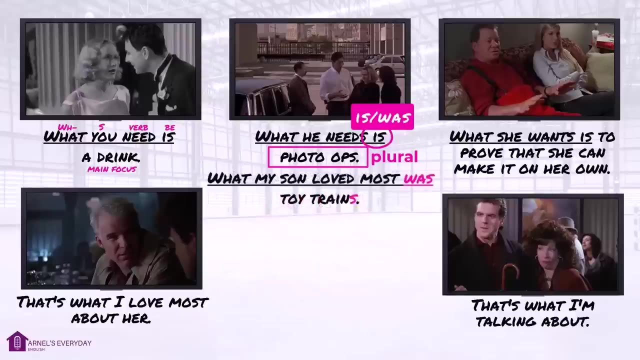 become more popular. Celebrities and politicians need photo ops. Hmm, photo ops is plural. Why do I have a singular verb? The WH clause is considered singular in clef sentences, So even if your noun is plural, use is or was. Here's another example: What my son loved most was: 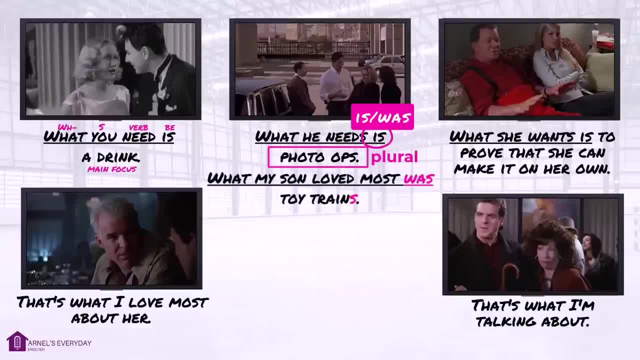 toy trains, Plural noun, but B stays singular. Yes, it's possible to use are and were, but that's considered less formal. In the third example, after B, we have an infinitive. So the main focus of a WH. 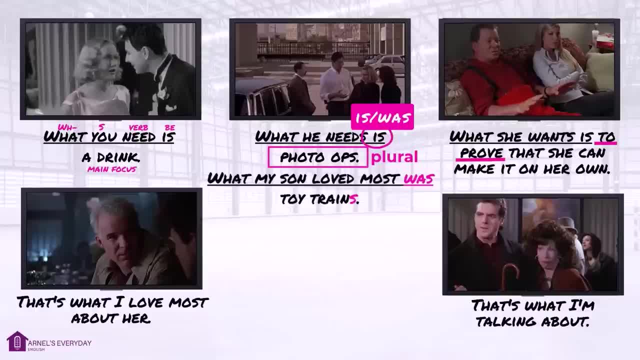 clef sentence doesn't have to be a noun. Remember what I said. There are lots of varieties. Look at these last two examples. These have already been reversed. What I love most about Annie is most about her. is that What I'm talking about is that Here that is acting as a pronoun, So 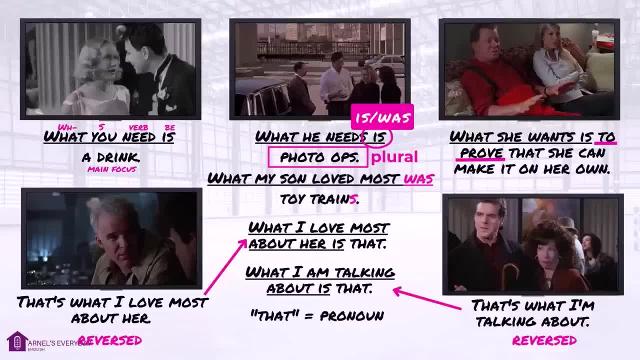 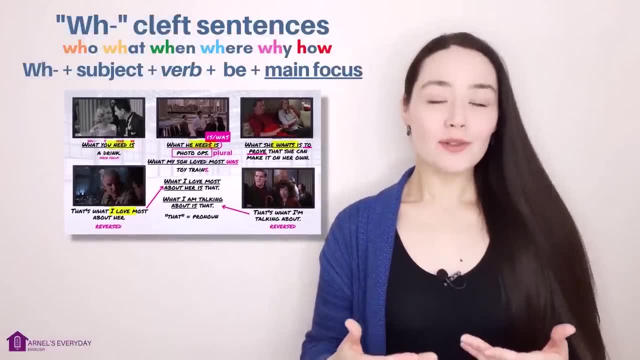 beginning a clef sentence with. that is really common. You might also notice the verbs need, want, love. A lot of times we use these emotional verbs. Okay, we've looked at quite a few clef sentences beginning with what, but of course there are other WH words. 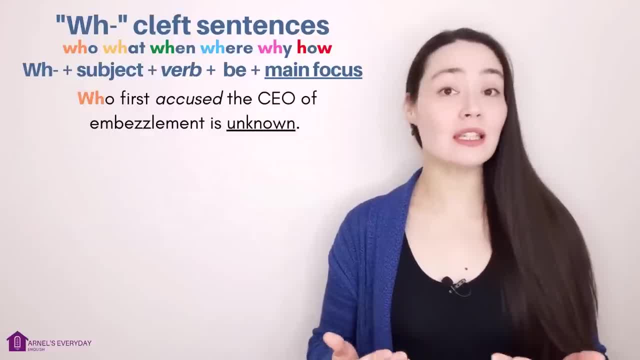 Are you joking, Jessi? Oh, one of you said That's my cue for making you stupid comments, right? The rest of the day isn't required and it's definitely not. Who first accuse the CEO of embezzlement is unknown. 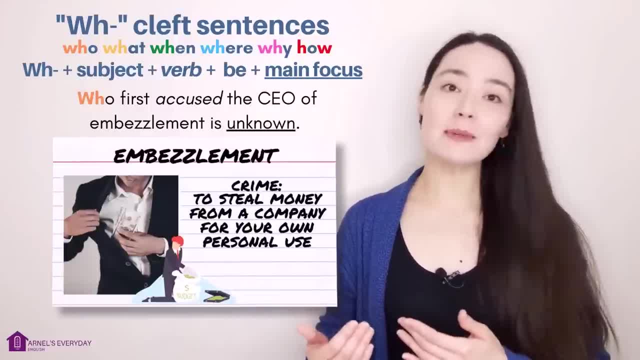 A good crisis Decision making. Who first accused the CEO of embezzlement is unknown. Embezzlement- Embezzlement is a crime. It means stealing money from a company to use for your own personal. When a person should get married is WA WASN'T SHOULD GET MARRIED is a personal. 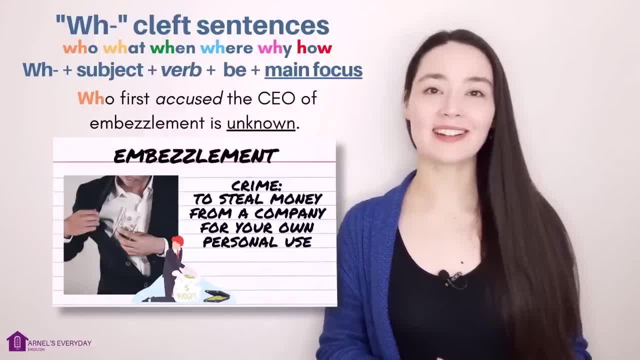 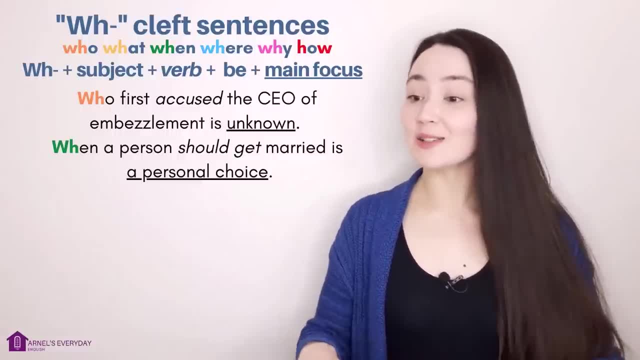 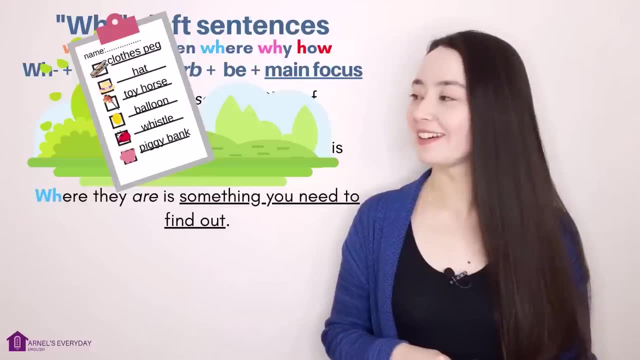 choice. A judge must have an accurate picture of when the woman in a present tense would say A Fa. the word very quickly: Fa b blah voted a Fa bleab woman in this park. Where they are is something you need to find out: What- where they are. 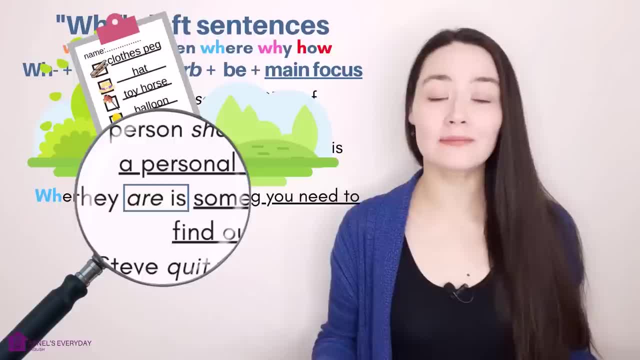 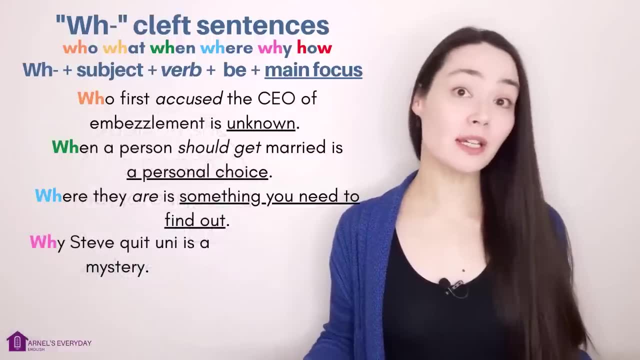 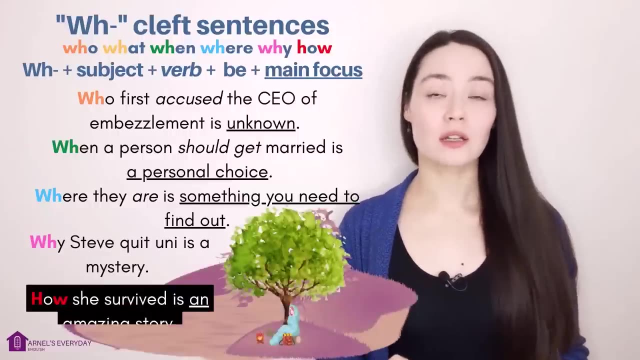 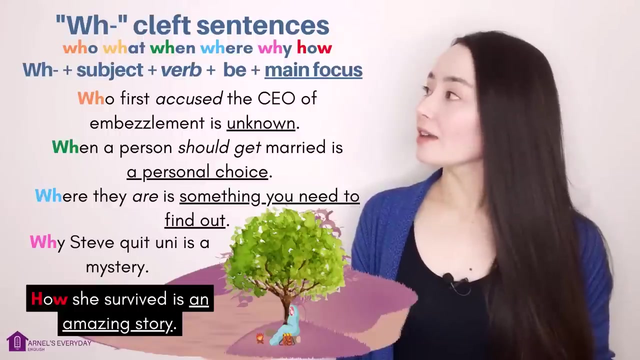 is: Is it possible to have a double B? Absolutely correct. Why Steve quit uni is a mystery. Sandra was lost in the woods for three weeks. How she survived is an amazing story. You should read her book. Okay, in this structure we can replace WH with. 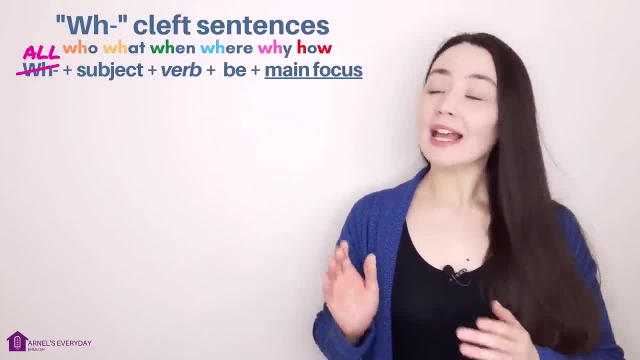 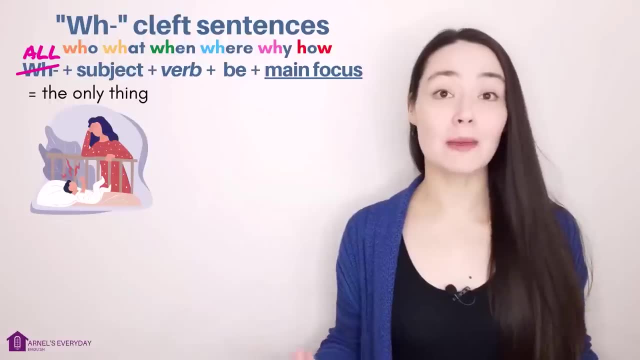 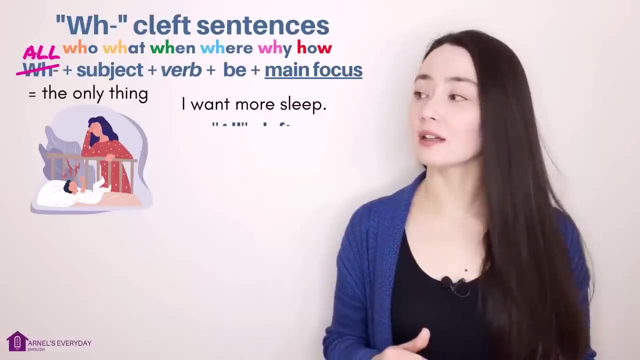 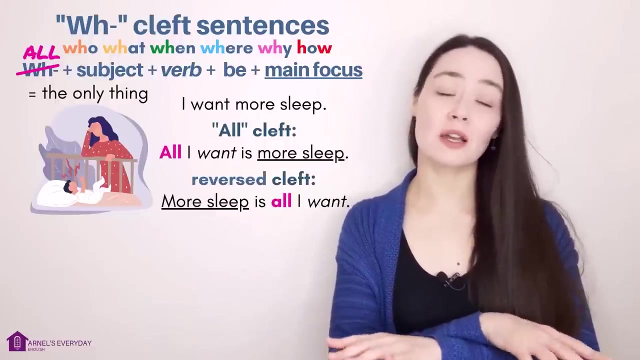 all. All is really common and in this case, all means the only thing. Imagine a parent with a new baby: I want more sleep. Standard sentence. Let's emphasize that All I want is more sleep. More sleep is all I want. These all clef sentences are really common in songs. 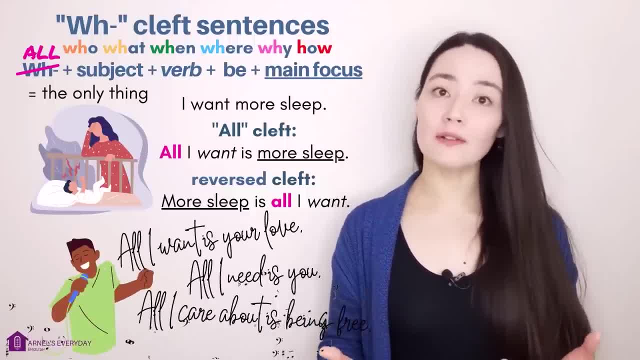 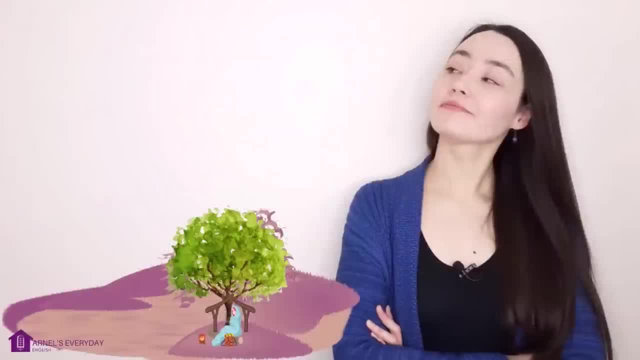 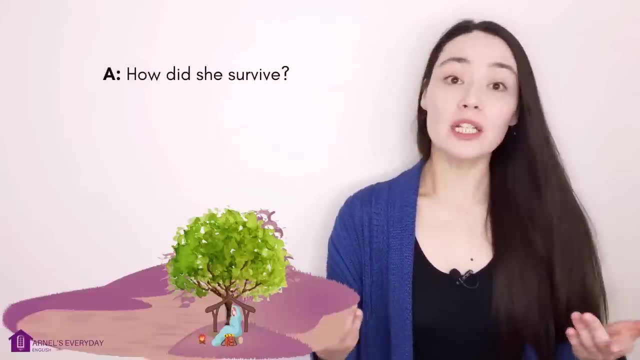 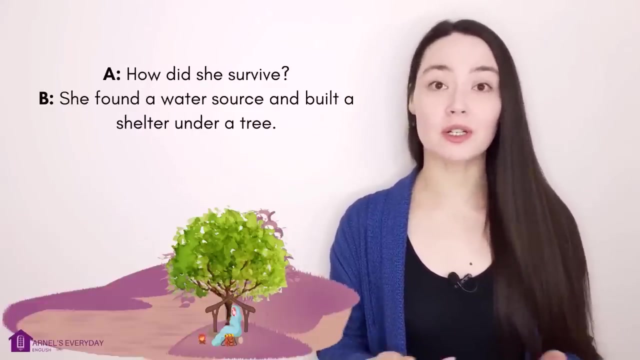 Why? Because songs are emotional, so a lot of times people try to add more emphasis by using this grammar. Remember how Sandra was lost in the woods for three weeks. How did she survive? Standard sentence: She found a water source and built a shelter under a tree. Now this is pretty. 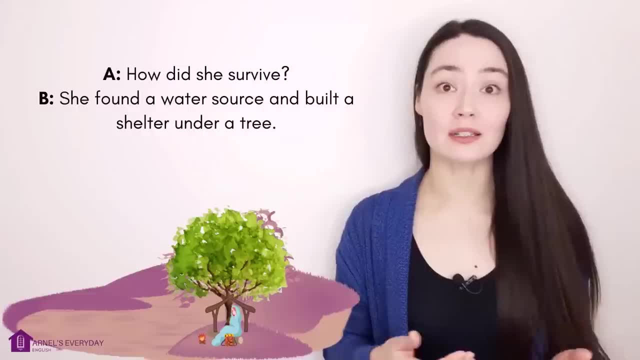 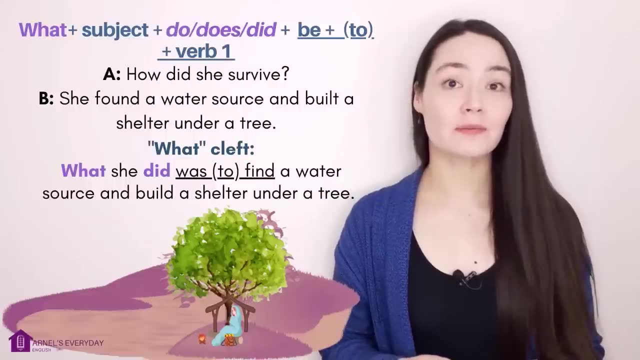 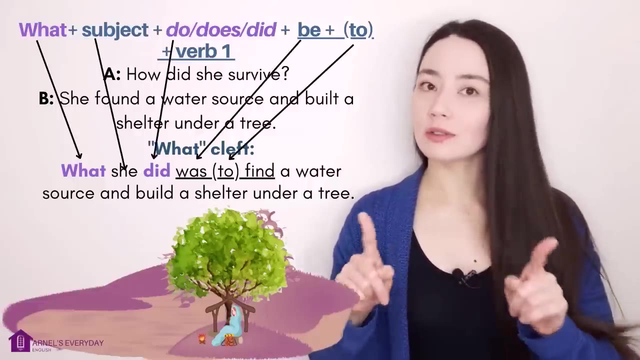 impressive. It's a great opportunity to use a clef sentence. What she did was find a water source and build a shelter under a tree. What Subject do, did, does be to is optional Verb one. It's quite a long structure, So we use this structure. 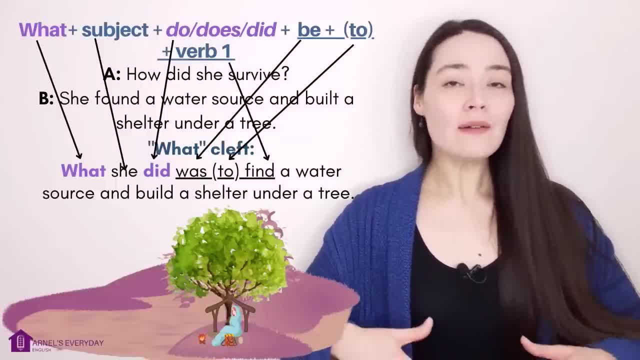 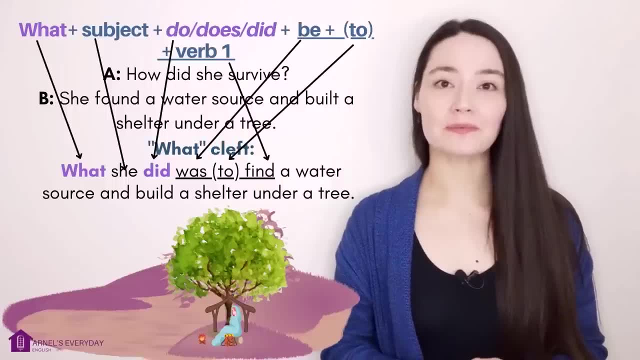 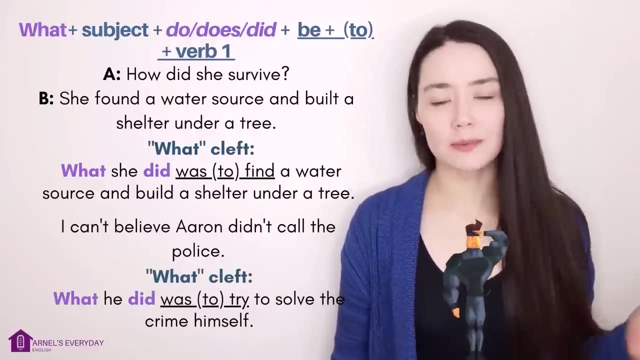 with do, did, does, when we want to emphasize an action, An action that has quite a bit of information connected to it. I can't believe Aaron didn't call the police. What he did was try to solve the crime himself. What Subject: do, did, does? 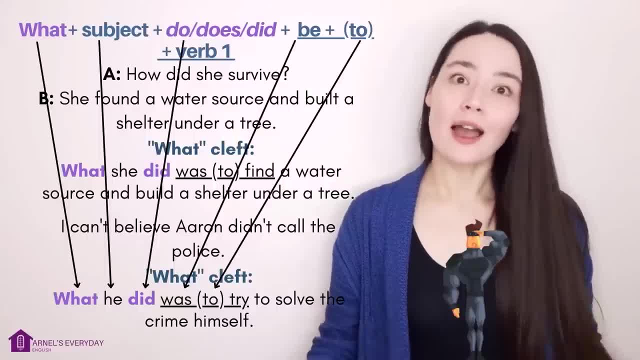 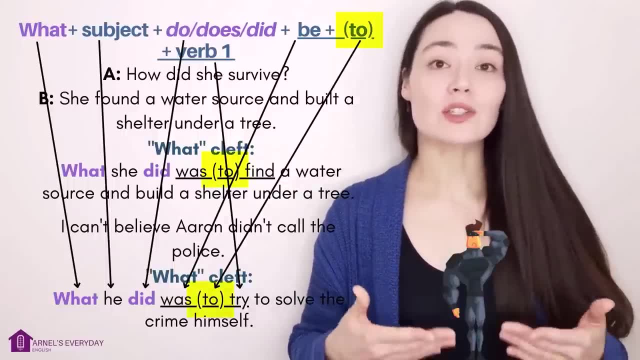 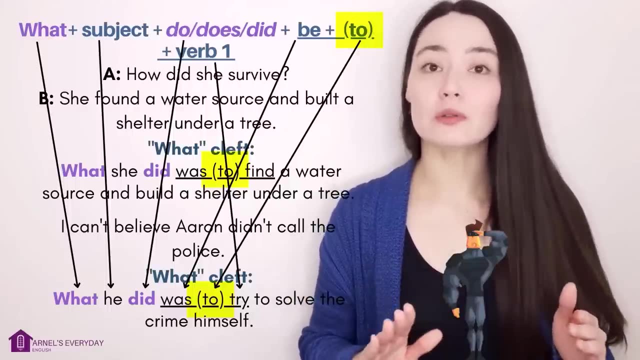 be to is optional and verb number one. So in both of the examples I gave you you can see to in parentheses. Yes, to is optional. You can choose to use it or not, But in my opinion the structure without to is more common And just like: 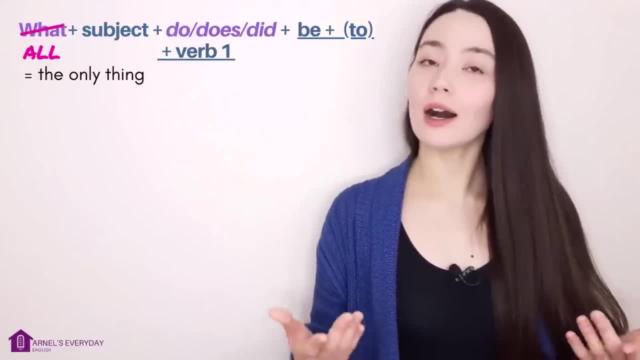 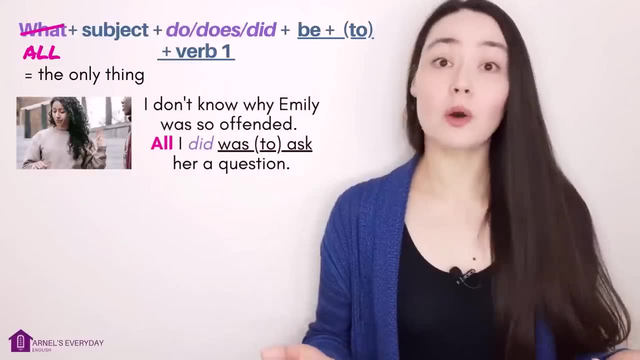 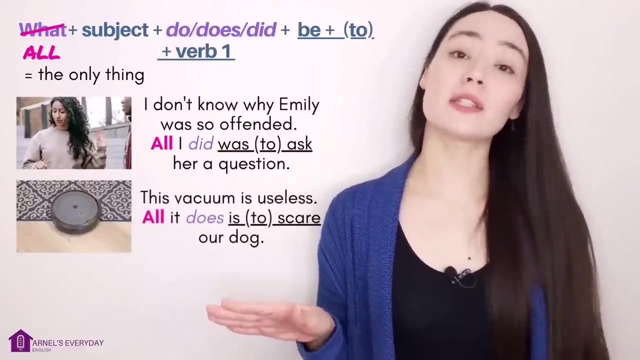 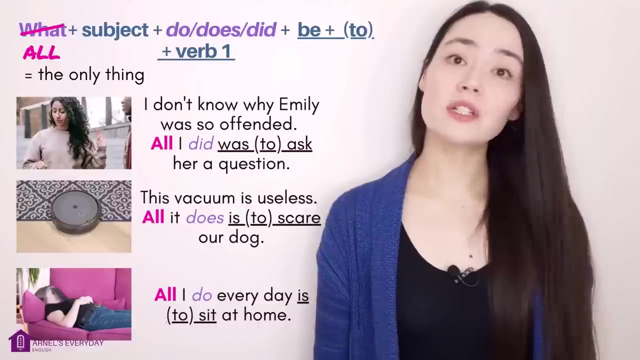 earlier. we can replace what with all. Again, all meaning the only thing. I don't know why Emily was so offended. All I did was ask her a question. This vacuum is useless. All it does is scare our dog. All I do every day is sit. 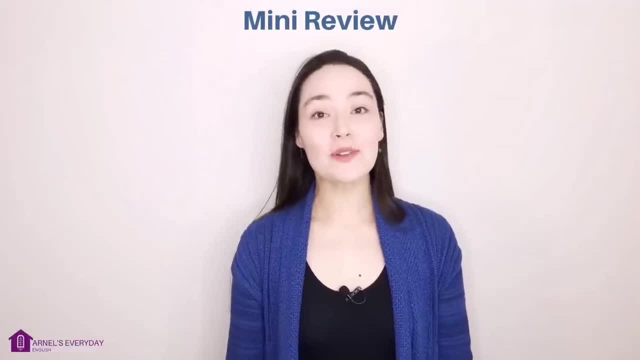 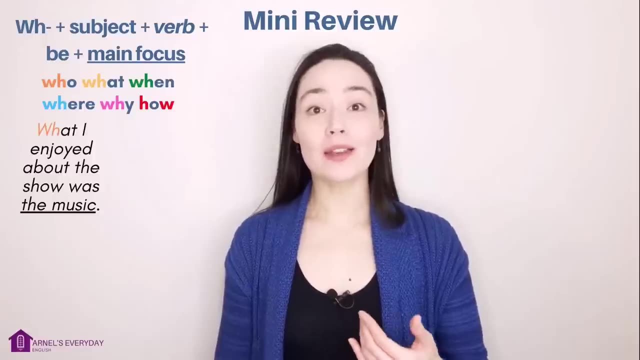 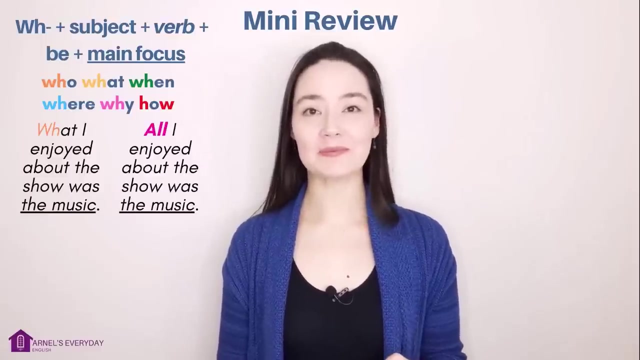 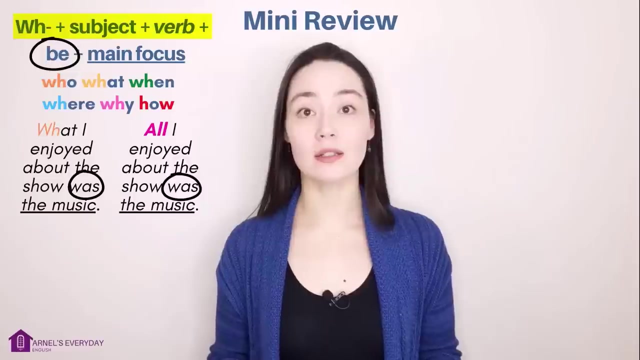 at home. Another mini review before the test. In this structure here we can use who, what, when, where, why and how. We can replace wh with all That's also possible. The wh clause is considered singular, so be is singular, Is or was. Sometimes you might hear are or were, but that's. 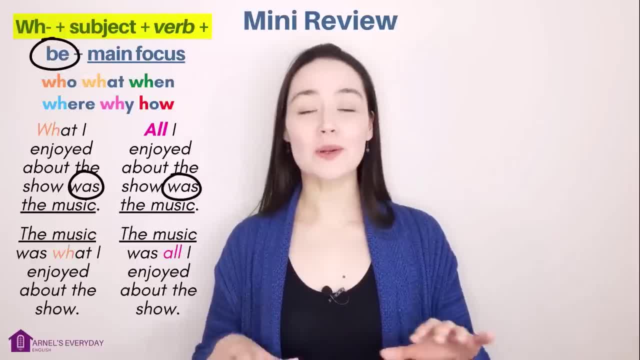 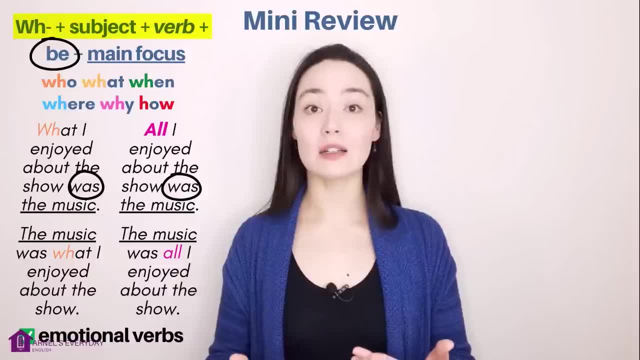 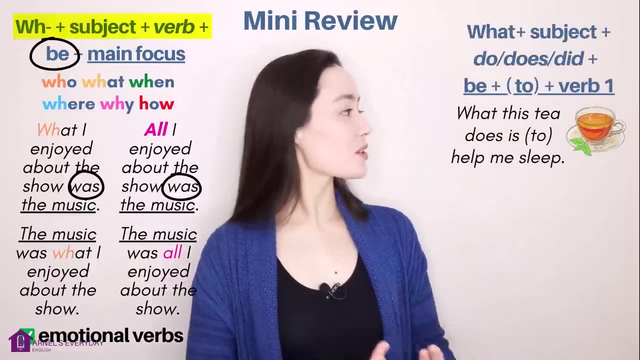 considered less formal. In this structure here we can reverse the parts Perfectly correct, And we often see emotional verbs like need, want, like love, enjoy, things like that. We also have this structure here We can replace what with all. 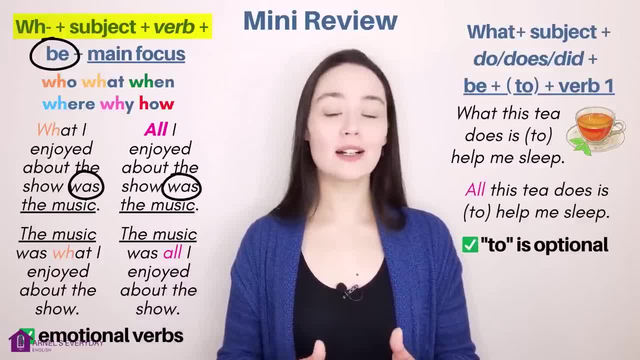 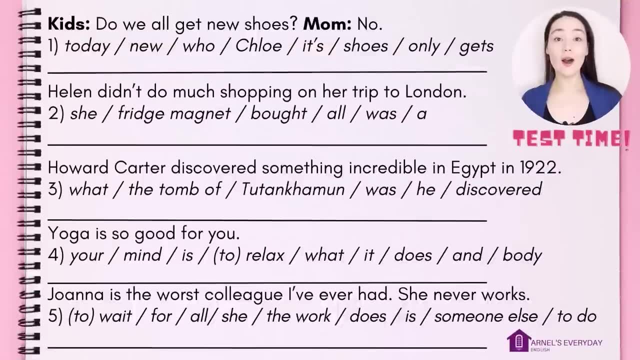 And here too, is optional. Okay, are you ready for a test? Okay, test time. One of the most important things to remember about cleft sentences is the structure. Without that structure, cleft sentences really don't work. So that's what I want. 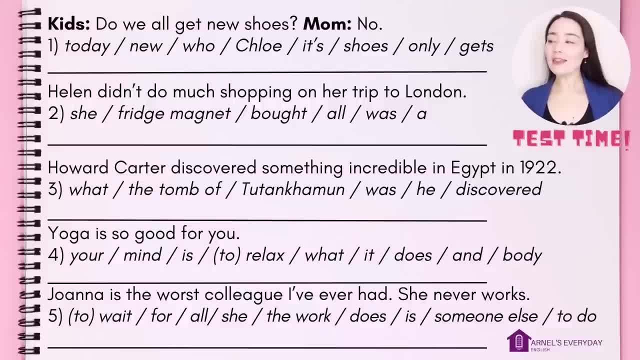 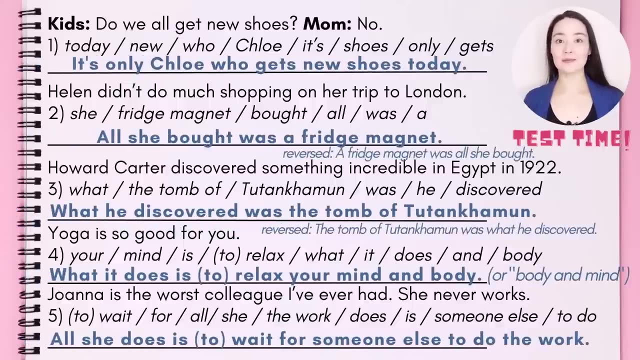 to test. I have five sentences and they have been scrambled up. Can you please, please, make complete sentences by putting the words in the correct order. Pause the video to do this Right. here are the answers And just so you know, in number one today can go at: